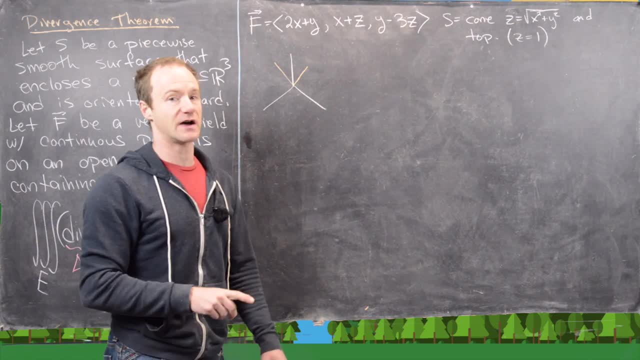 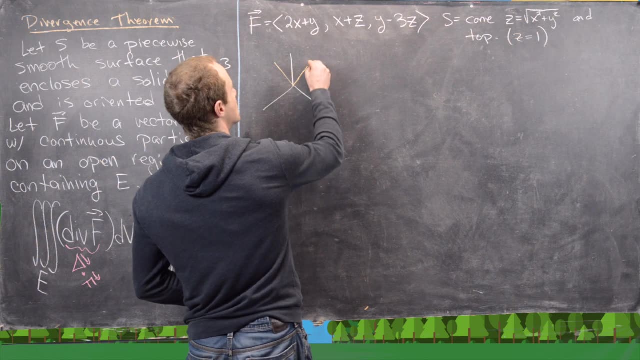 So this looks like it's opening in a flat way, like the absolute value functions do, Okay, And then it opens circularly, if you're looking down on it, Okay, great. So let's see, We've got this kind of picture right here. 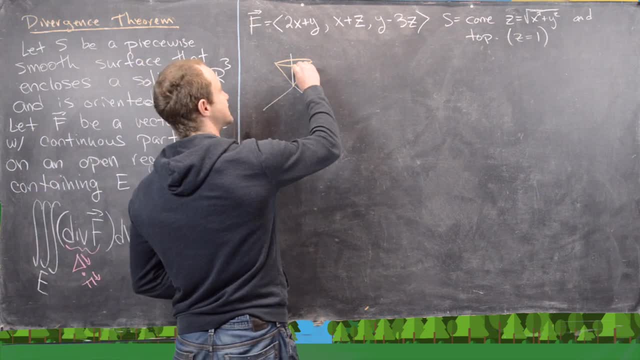 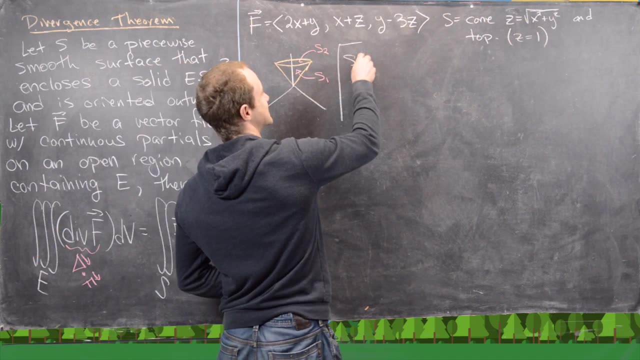 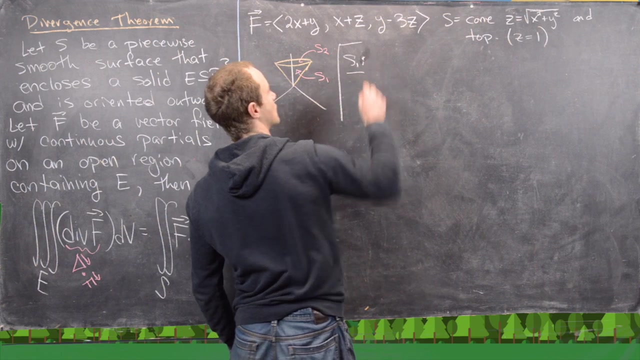 So that's our cone. Maybe we could call these sides here s1, and then we'll call the top s2.. Let's go ahead and parametrize the side first, in other words s1,, and I want to do that by taking inspiration from spherical coordinates. 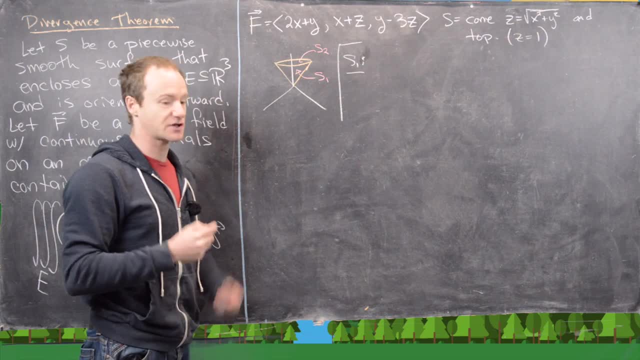 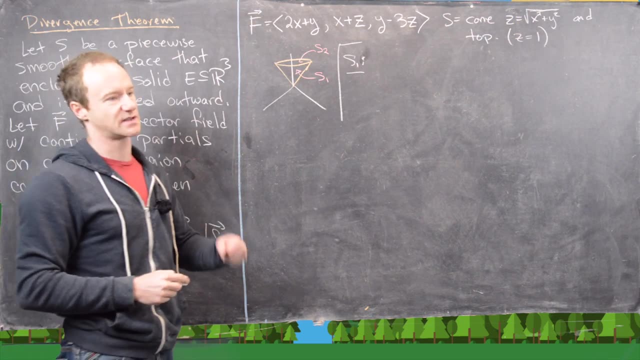 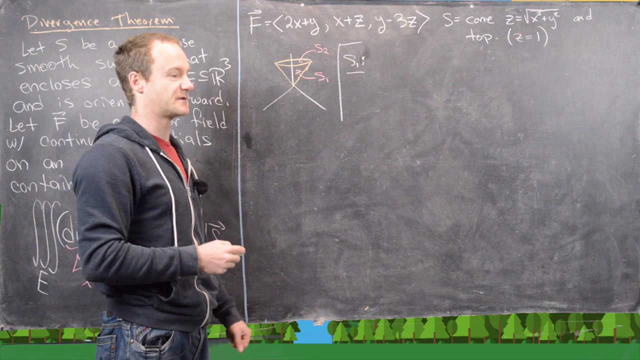 And often, whenever we're wanting to parametrize these surfaces, you can take inspiration from some coordinates system which is quite common, like spherical coordinates, cylindrical coordinates, so on and so forth. So, as we'll see in this example, we'll parametrize one with inspirations from spherical coordinates and the other one being inspired by polar coordinates. 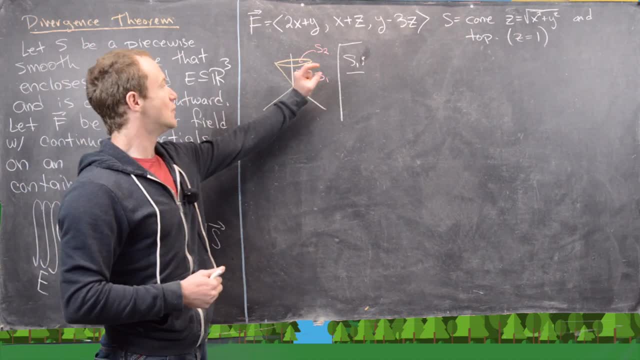 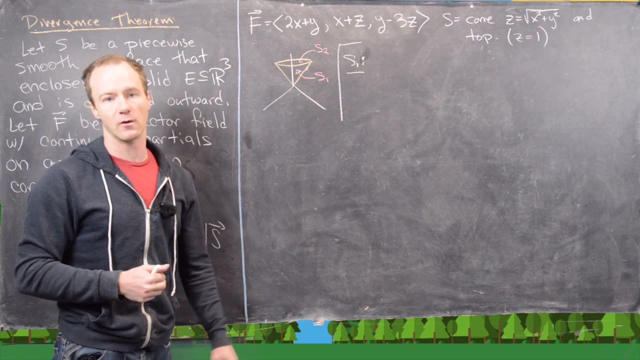 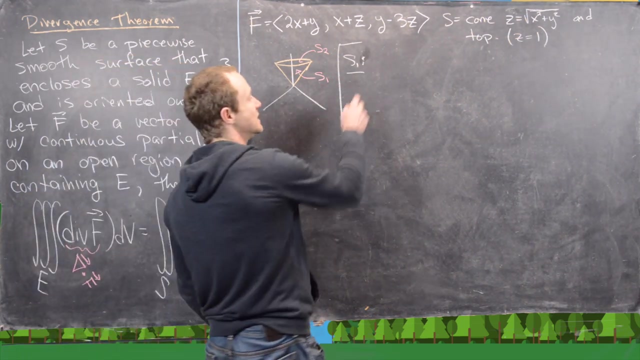 So here we'll take spherical coordinates, because we know that this cone has a really nice formula in spherical coordinates, and that is: phi equals pi over four, and you can see that because it's halfway between the positive z axis and the xy plane. okay, great. so spherical coordinates are given by rho. 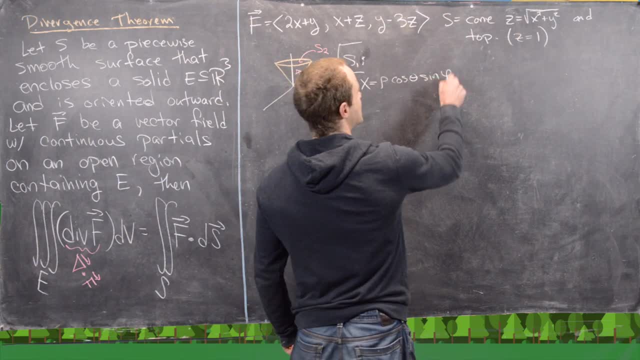 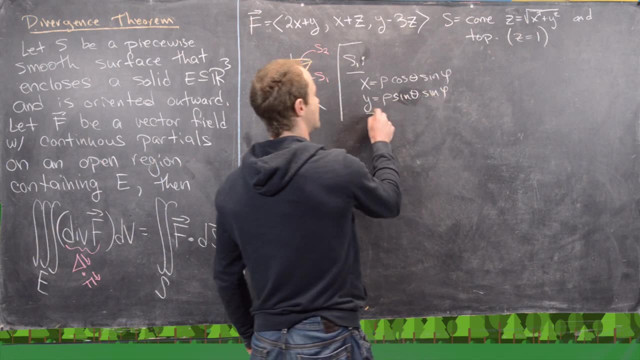 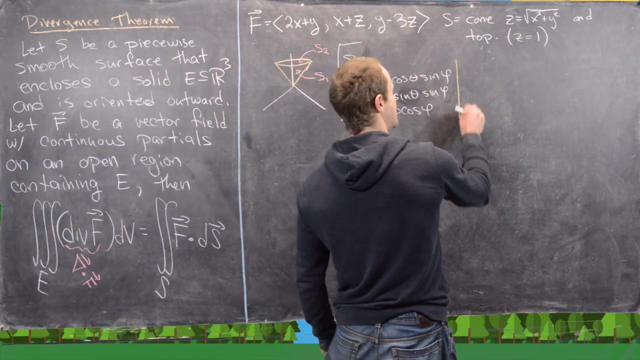 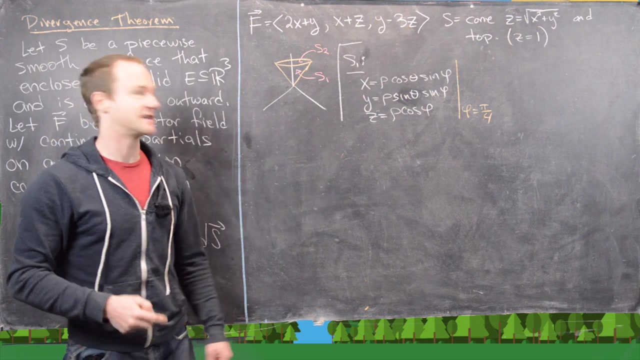 cosine theta sine phi. y equals rho sine theta sine phi. and then, finally, z equals rho cosine phi. and, like I said, if we set phi equal to pi over four, that puts us right on top of that surface, or I should say right on the sides of that surface. 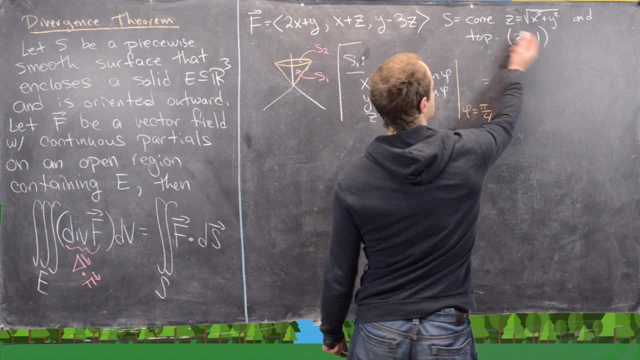 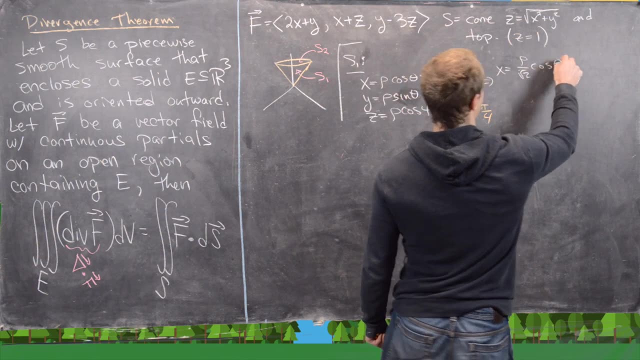 so that is going to give us a row. so that's going to give us: x equals rho over root, 2 times cosine theta. that's because sine of pi over 4 is 1 over root 2, or root 2 over 2, if you. 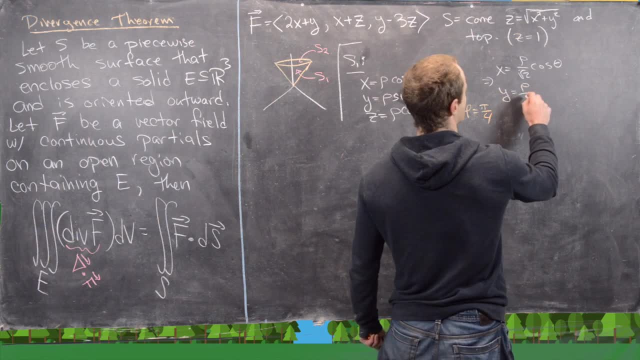 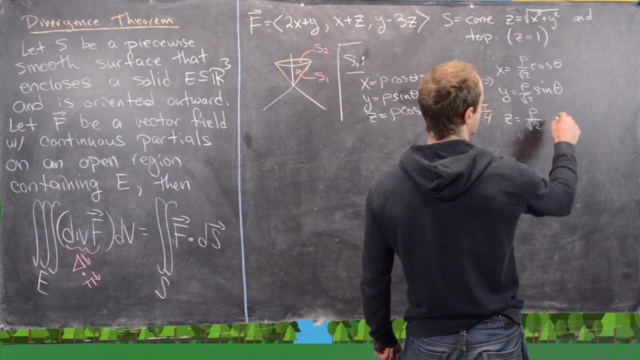 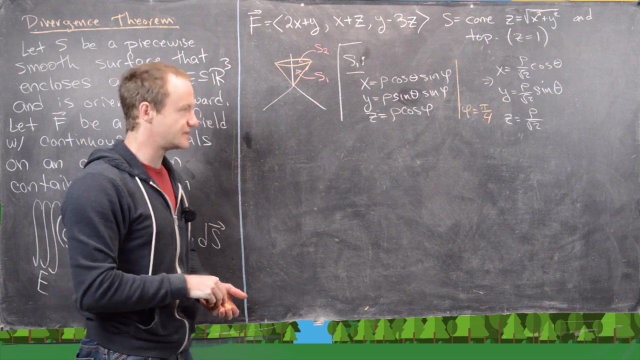 want to rationalize that denominator that gives us y equals rho over root 2, sine theta, and then finally that gives us z equals rho over root 2, and then that's it great. but now we can actually simplify this quite a bit and we can do. 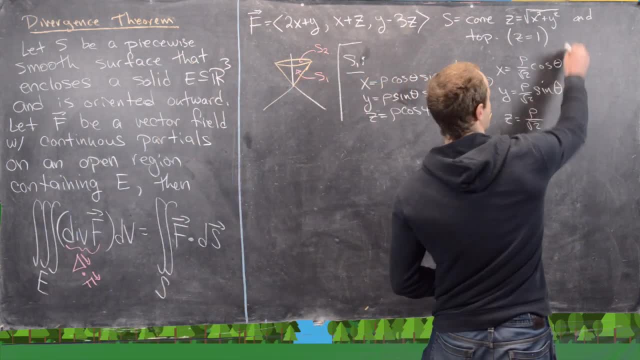 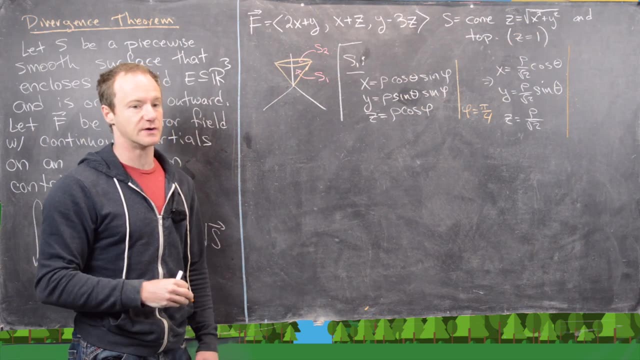 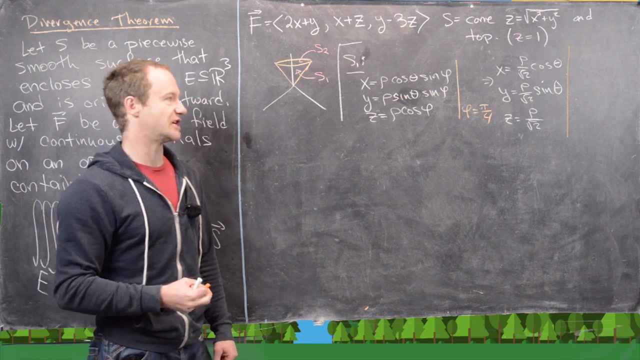 that by making a slight change of variables- and this is also something you might want to do after setting one of your parameters in your spherical coordinates or whatever equal to a number, in order to get on a surface- you might want to simplify the parameters afterwards by making a change. 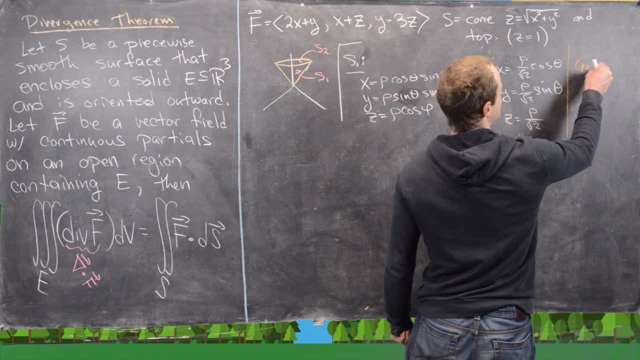 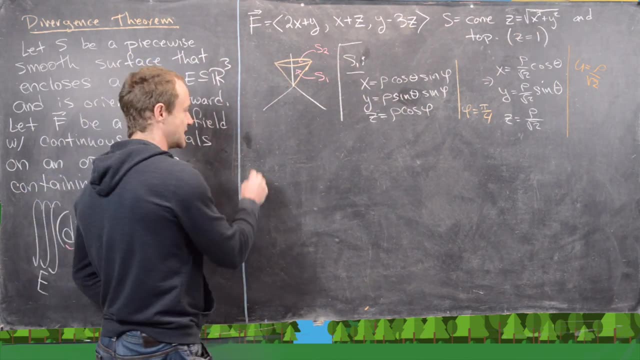 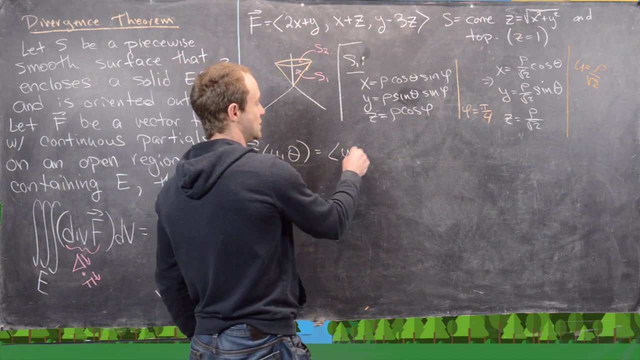 of variables. so here we might as well let u equal to rho over the square root of 2, because that ends up being inside of this all the time and that's going to give us a nice parameterization in terms of u and theta, and that is going to be u. 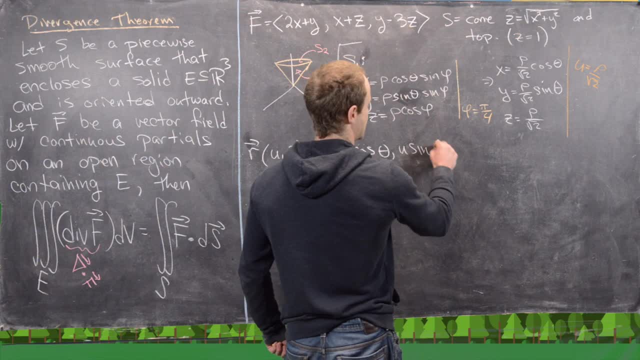 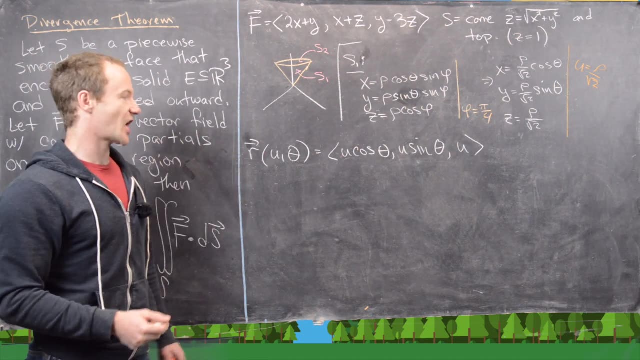 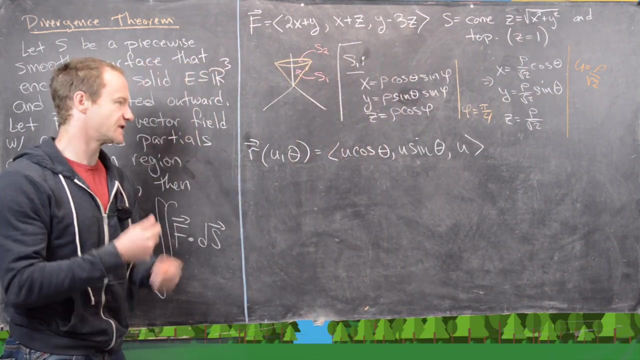 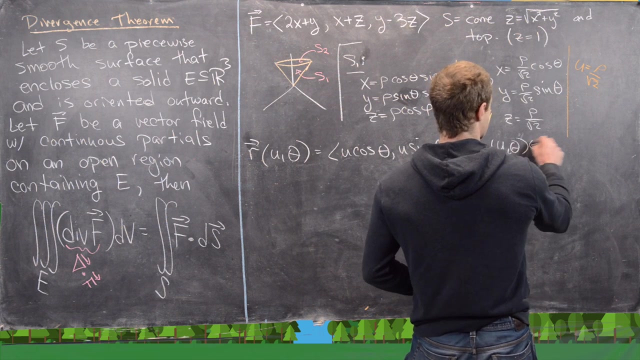 cos theta, u sine theta and then u. great, and now, now you can check that if you plug this x, y and z value into the cone, it actually satisfies that equation of that surface. so this is a parameterization. and now let's see what we need. we need u and theta to be on the 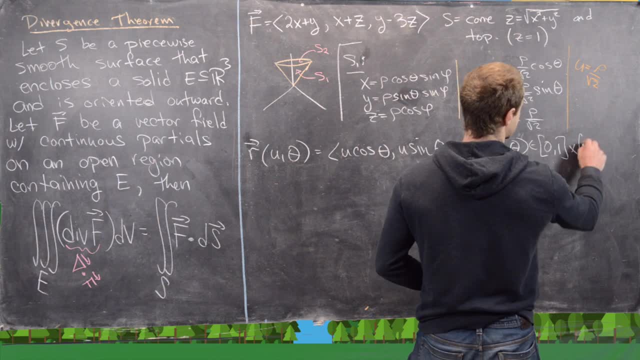 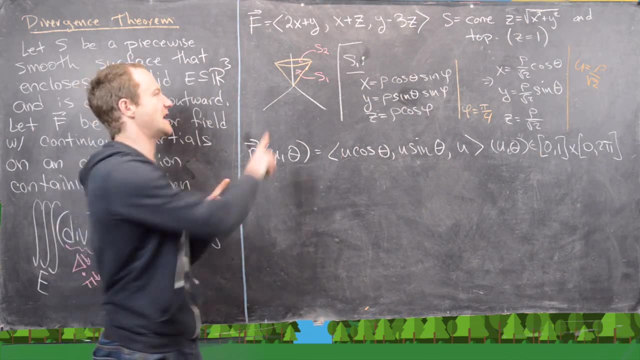 cross product of the intervals 0- 1 cross, 0 to 2 pi. so how do we see that? well, the theta going from 0 to 2 pi is because you need to trace out this whole circle which is making the cone and then the u. 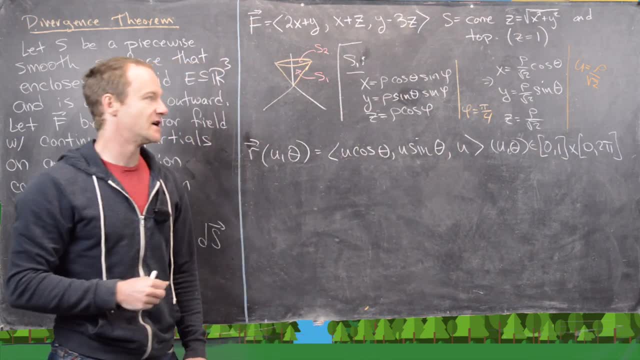 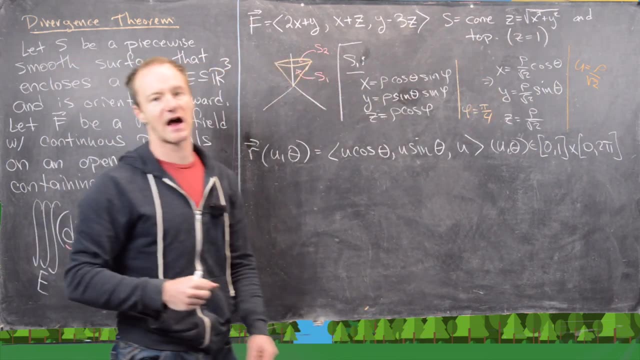 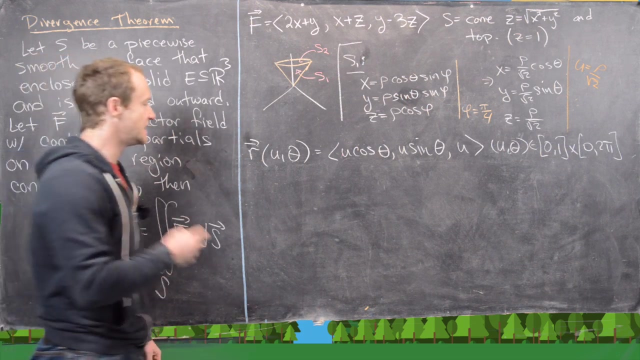 going from 0 to 1. it is because- notice- our z component is exactly equal to u, but our z component needs to go from 0 to 1, given that the top of our cone is at the z equals 1 axis. okay, great, so that's the parameterization. now the next. 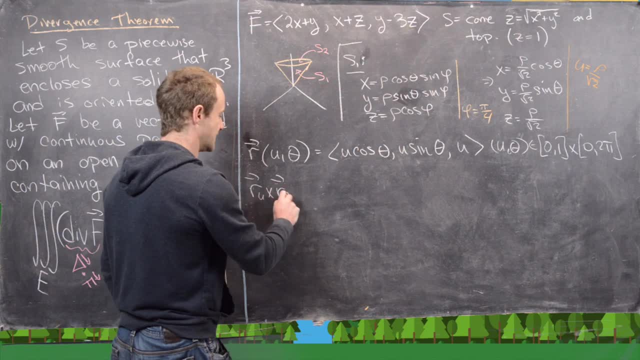 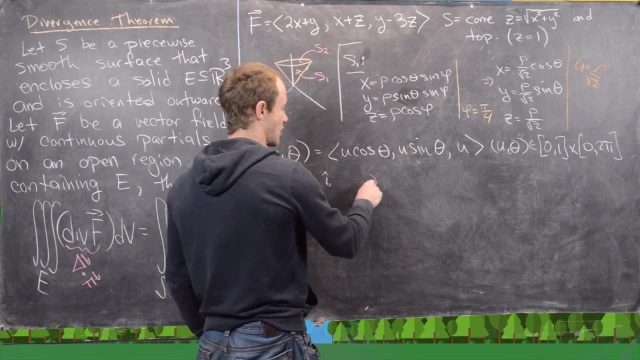 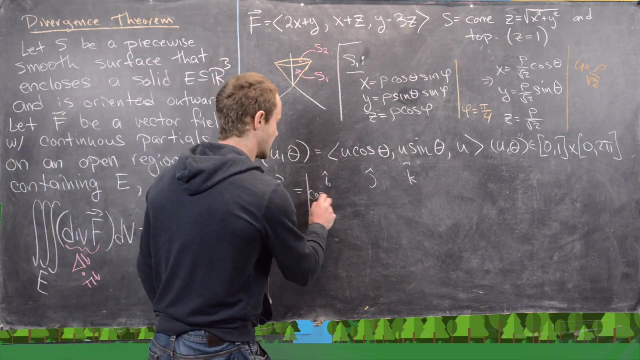 thing that we need is this: R? u cross, R theta, so that plays the role of this normal vector in the surface interval. so that means we're going to need to calculate the cross product of these two partials. so let's see: if you take the partial with respect to u, we'll get. 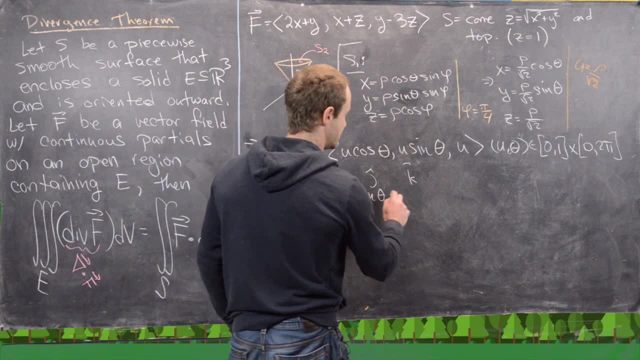 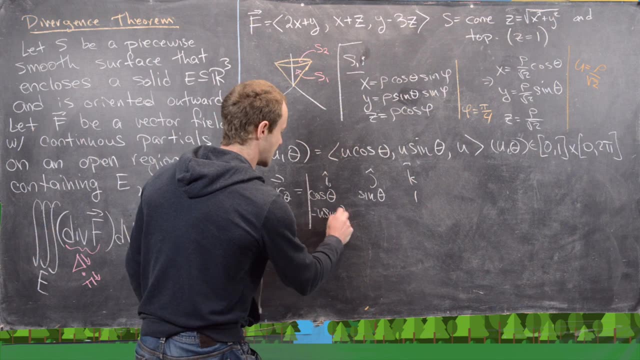 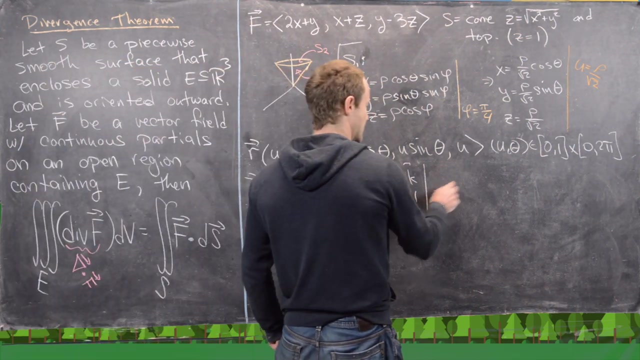 cosine theta sine theta, and then 1. if you take the partial derivative with respect to theta, we'll get minus u sine theta, u cosine theta and then 0. okay, great, but let's see what we get. so if we cross out the first column in the first row and then take that, 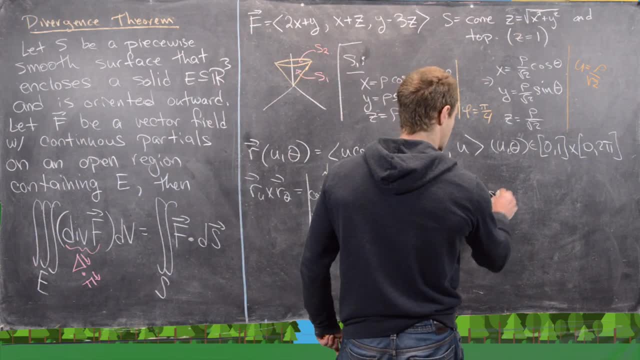 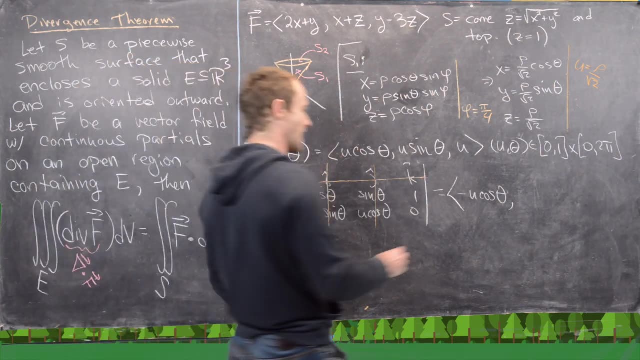 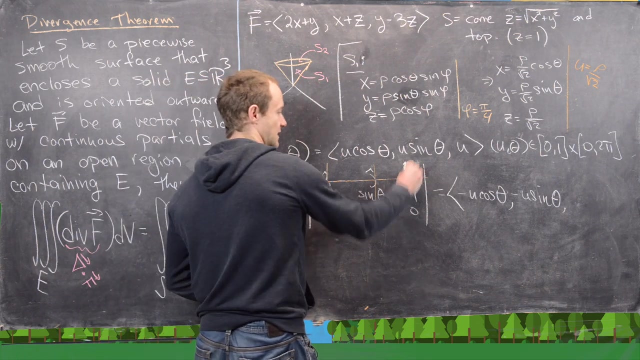 determinant, we'll get minus u cosine theta. then if we do the same kind of thing for the second column in the first row, we'll get minus u sine theta. and then, if we do the same kind of thing for the last column and the first row, we'll 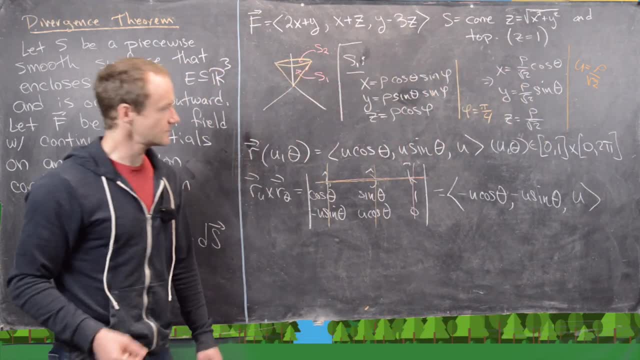 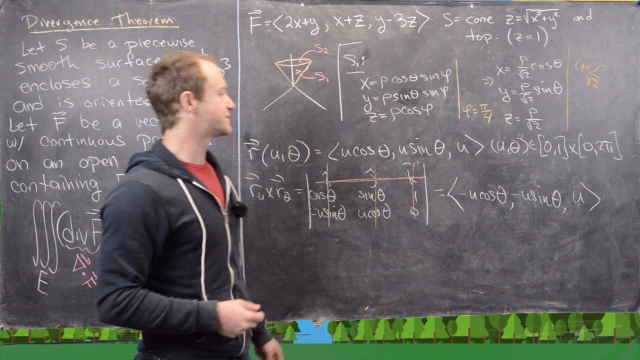 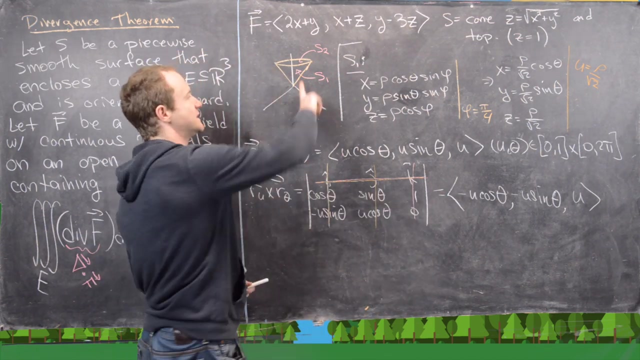 get u great, but if you see, this is a, this is actually pointing in the wrong direction. notice that here u is pointing. so notice, here the z component is pointing up and these are pointing inward. so this is actually an inward pointing normal vector, which is a problem because 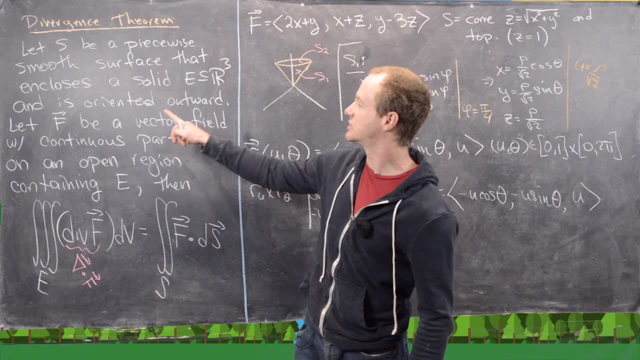 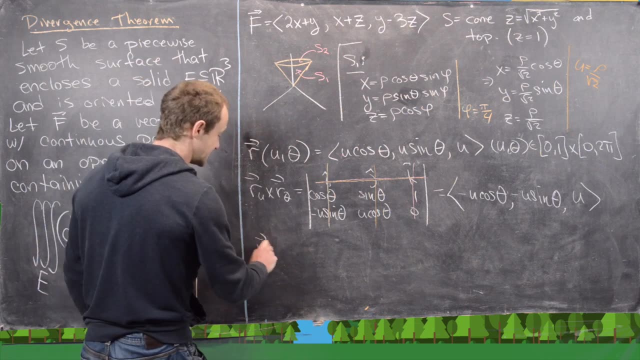 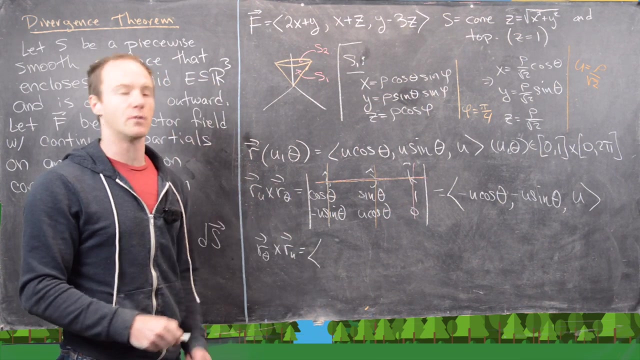 the divergence says that our surface needs to be oriented outward, but luckily we can change that just by taking, instead of R? u cross R? theta, we'll take R? theta, theta cross R? U to be our normal vector. We're calling that. when you change the order. 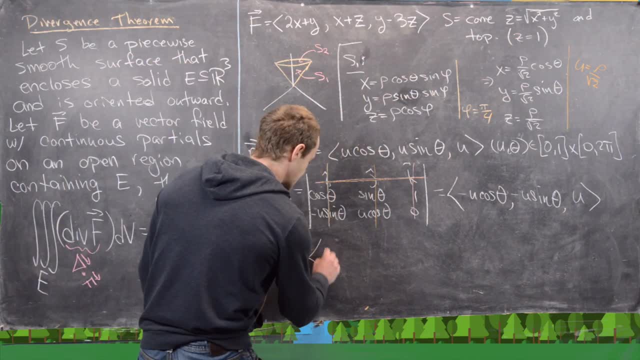 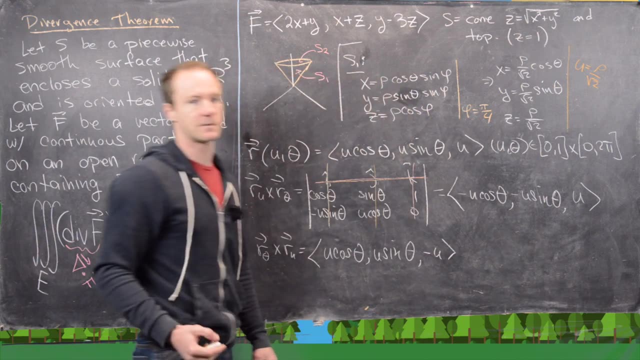 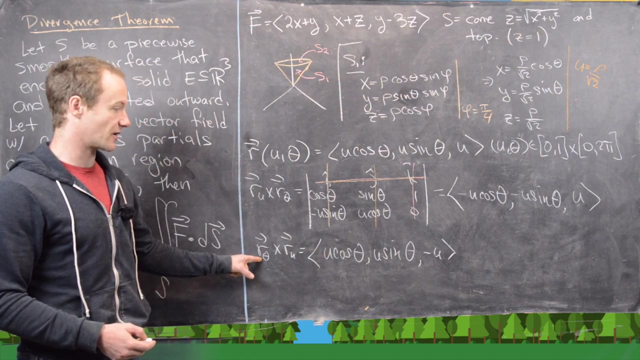 of a cross product. you just get a minus sign. So this is gonna give us U cosine theta, U sine theta, and then minus U, And that will be an outward facing normal from this S one. Okay, so that's what we need here. 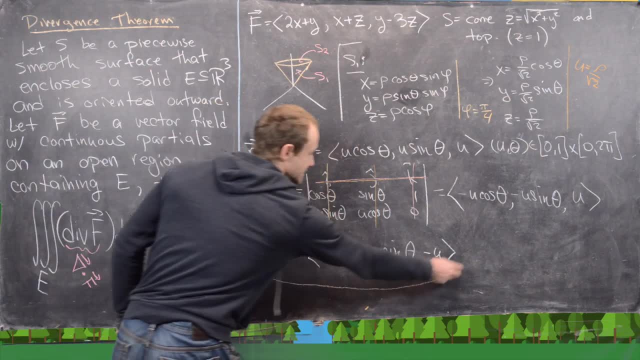 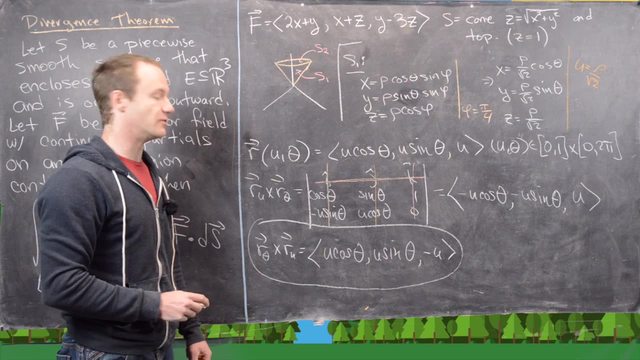 So the next thing we need to do is use this to plug into the formula for the surface integral. So I'll go ahead and clean up the board and then we will move on from there. So on the last board, we built this parameterization. 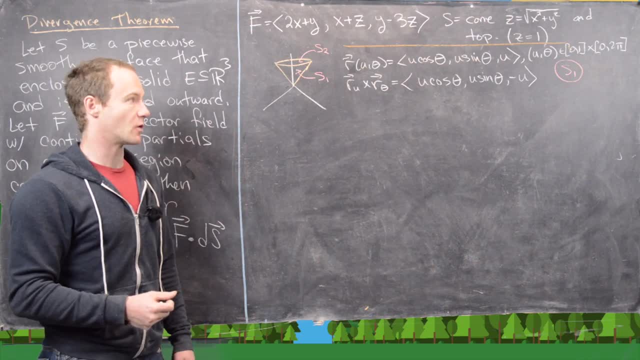 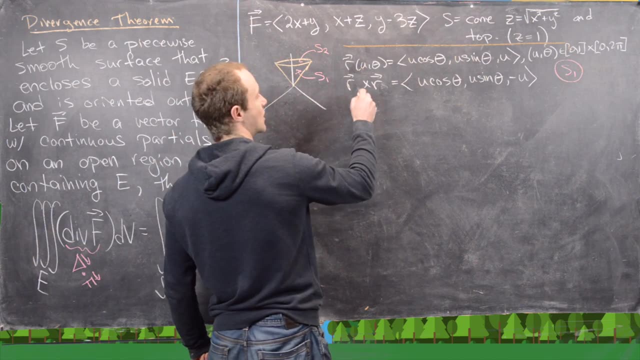 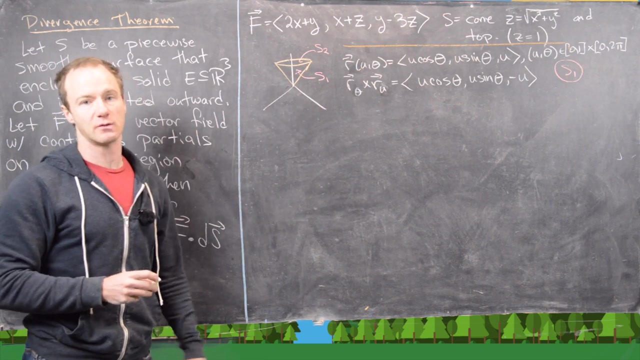 for our cone, out of inspiration, by spherical coordinates, And then we calculated this R? U cross R? theta And I should say we took this to be R? theta cross R? U. We took the different ordering of this And this parameterized this thing that we're calling S one. 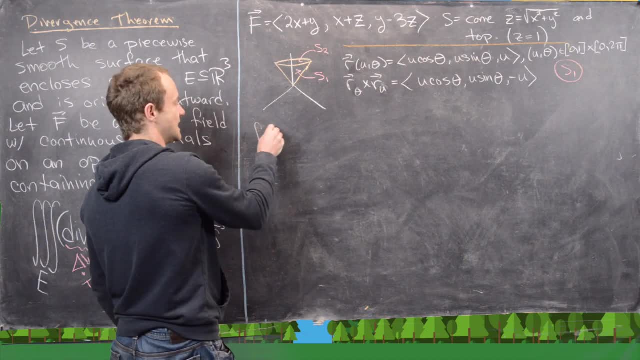 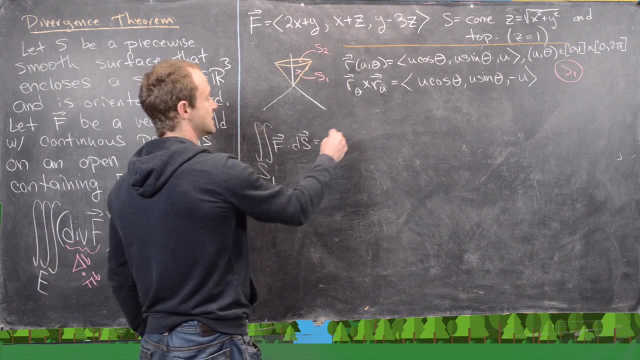 which, like I said, was the cone. Now we can go ahead and take the surface area over this, So the surface area over S one of F dot D S. So that's going to be the integral from zero one, the integral from zero to two pi. 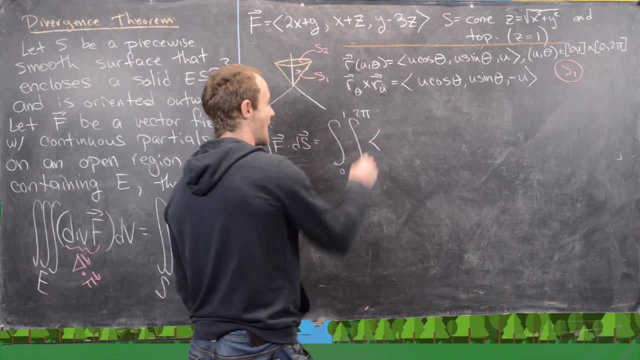 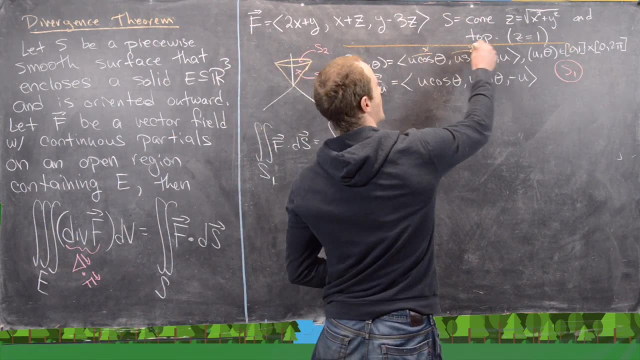 So we've got that iterated integral. Now we're gonna take F, evaluate it on the surface, which means we're gonna change all of the X values to this, all of the Y values to this and all of the Z values to this. 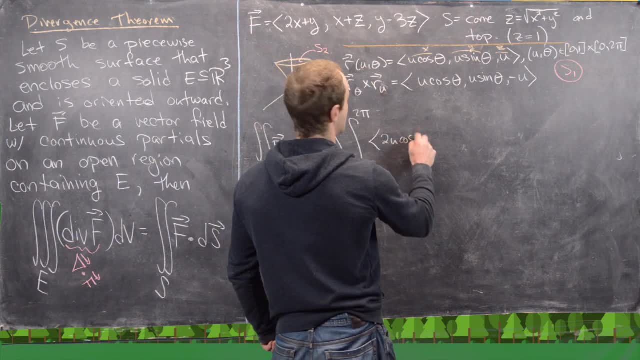 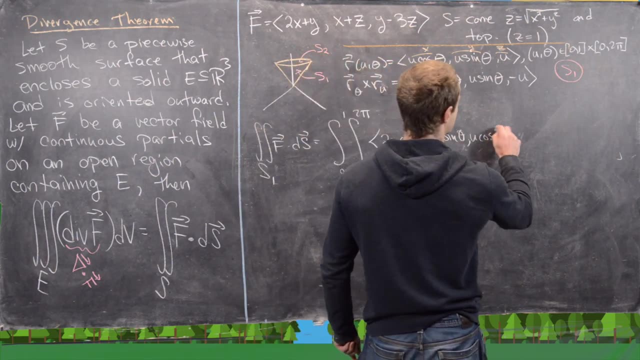 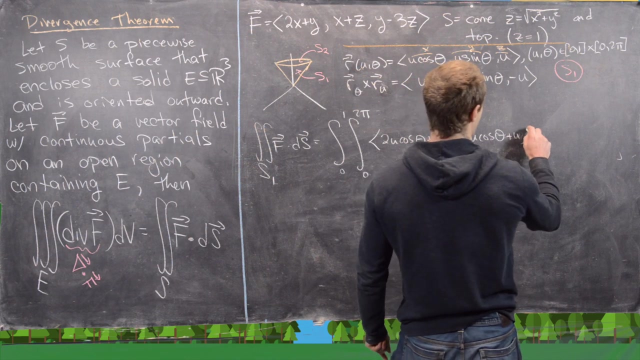 So that's gonna give me twice U cosine theta plus U sine theta. So that's my first component. And then I have U cos theta minus U plus U. That's my second component. And now I have U sine theta minus three U. 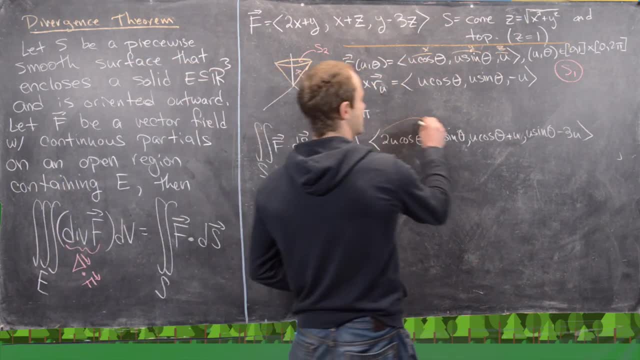 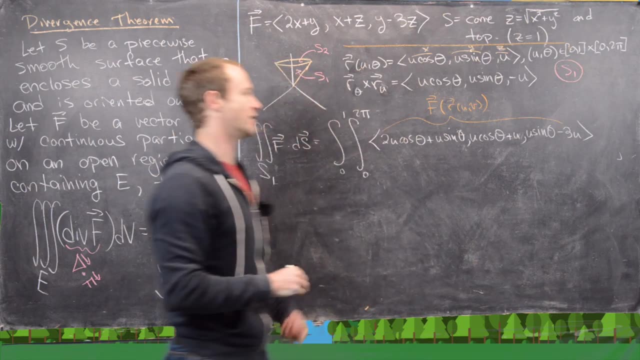 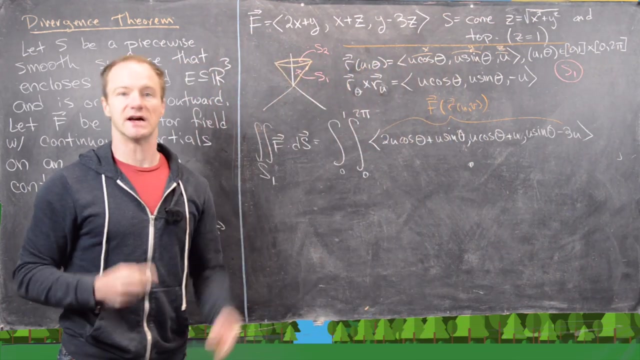 That's my third component. Just to reiterate, this is equal to F, our vector field, evaluated on our, on our surface. So F R U V. And now we need to dot that into this cross product. Again, this is built off of the formula. 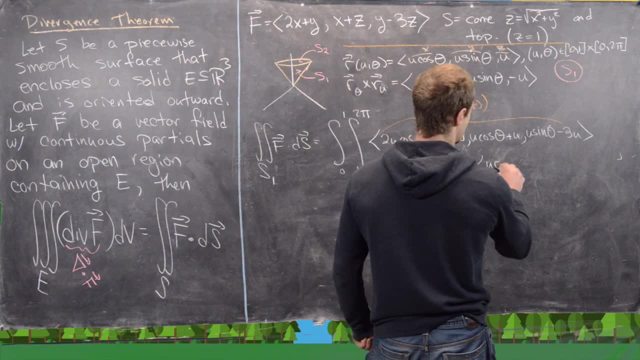 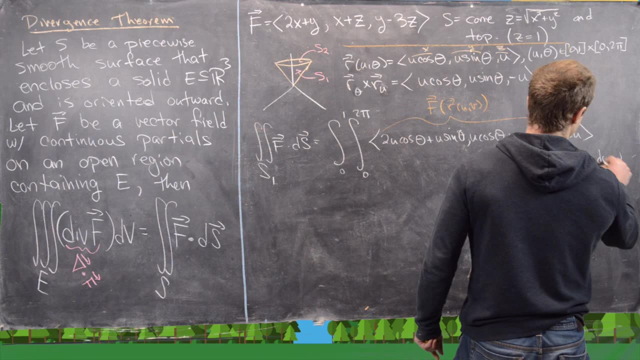 for the surface integral. So check that out if you need to. So here we have U cos theta, U sine theta and then finally minus U, And then we've chosen to do this in the D theta- D U order, Although, as you see here, 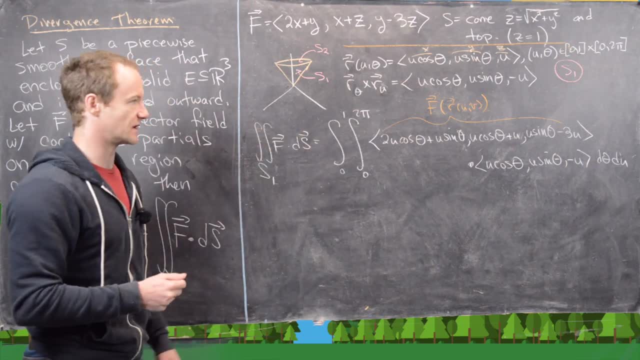 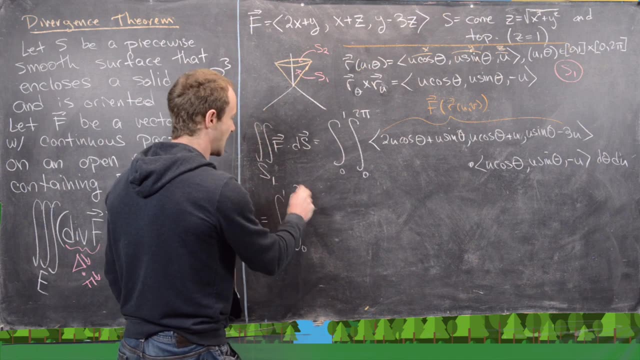 we can switch the order pretty easily because we've got- we've got nice bounds of integration and stuff like that, Okay. So let's see what we get for this. So we'll have the integral from zero to one, the integral from zero to two pi. 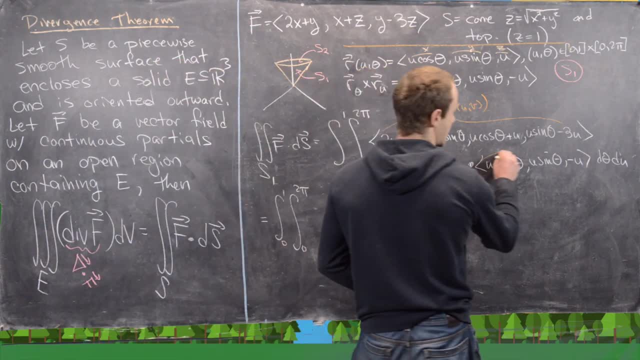 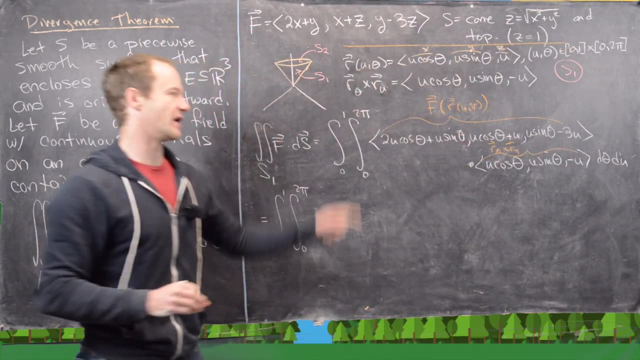 Now we need to do this dot product carefully. Before we do that, let's just recall that this part was R, theta cross R U. So our formula is F, evaluated on the surface, dot, that thing that we formed from taking that cross product. Okay, 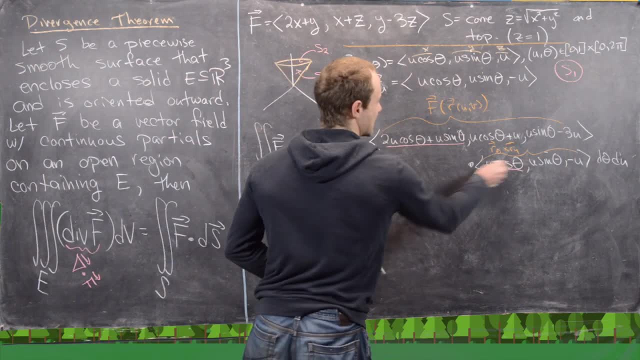 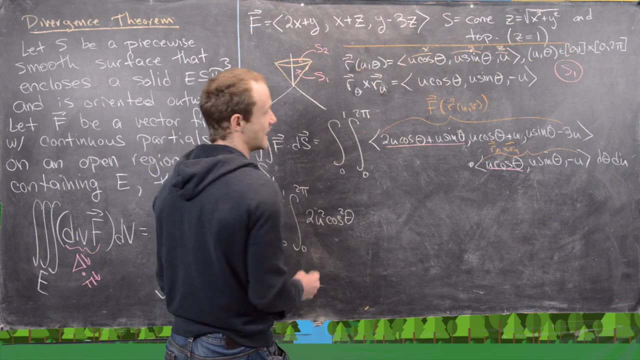 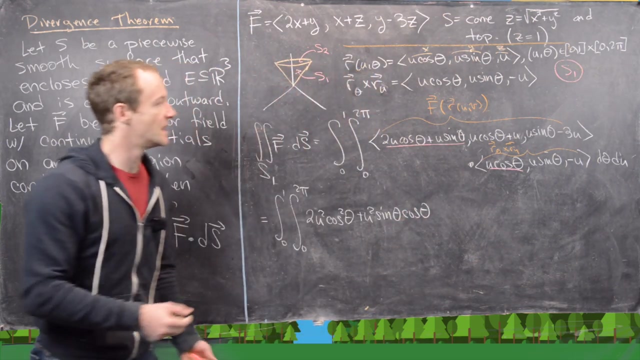 So let's see what we get. We need to multiply this with this for the first part of our dot product, So that'll give us two U squared cos squared theta, and then plus U squared sine theta cos theta Great. So the next thing that we need to do, 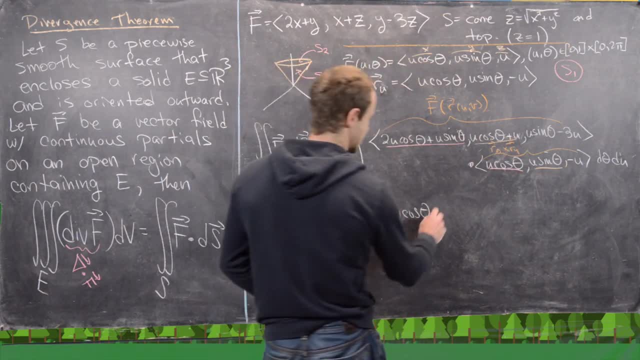 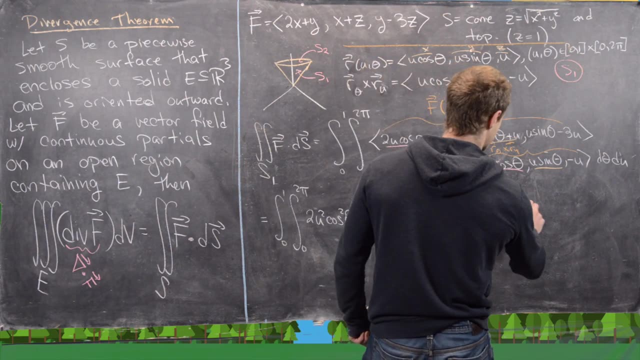 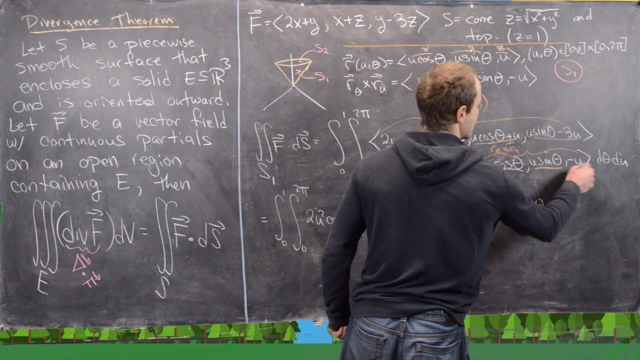 is: multiply this thing with this thing, So that's gonna give us plus U squared cos theta sine theta, and then plus U squared sine theta- Okay, great. And then finally we need to multiply that with that, And so that is going to give us: 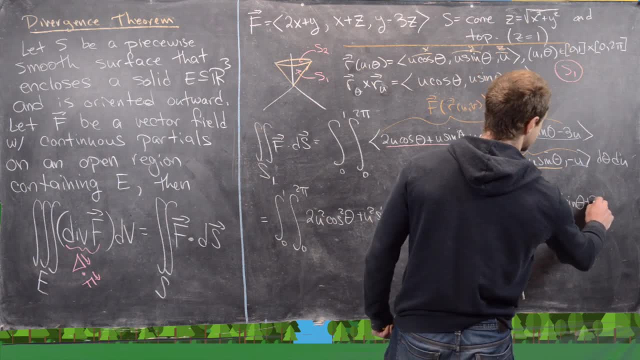 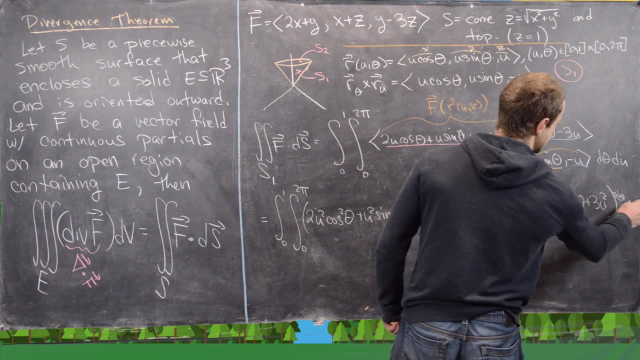 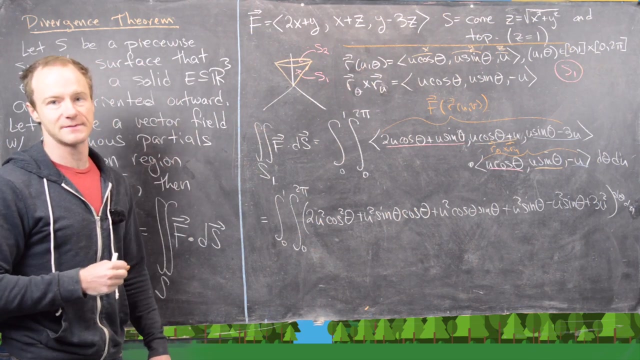 minus U squared sine. theta plus three U squared Great. And then we've chosen, like I said, to do this in the D theta D U order. Okay, So now I'm actually gonna skip a couple of steps here, because they're quite straightforward. 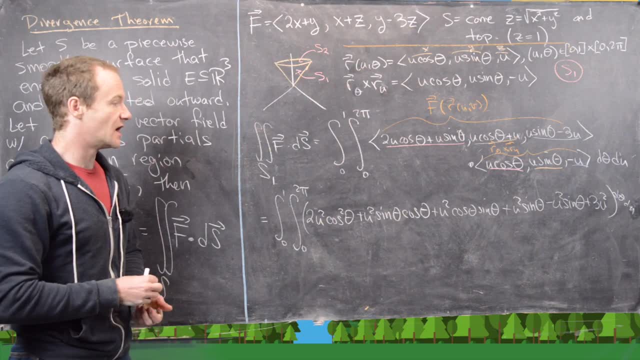 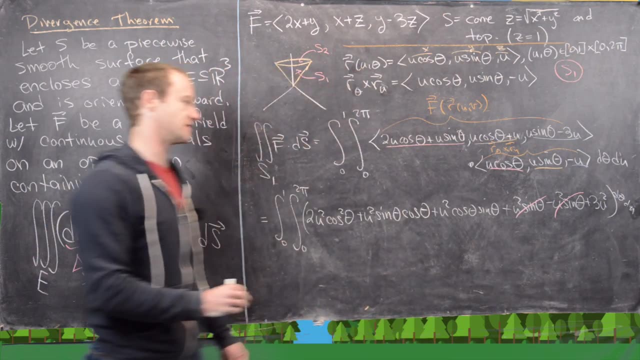 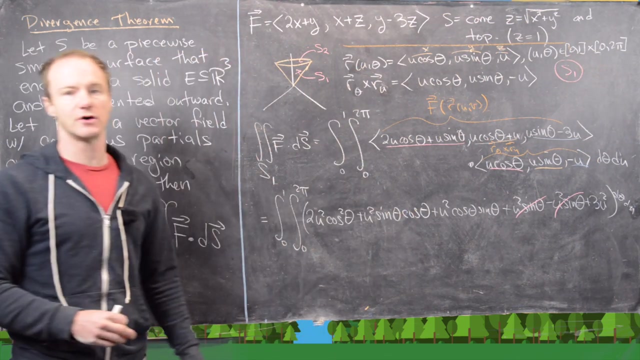 especially, kind of at the end of a calculus three class. this should be, um good, Pretty easy. So first of all, we can see that this sine and this sine cancel. And then the next thing that we can see is when we take the antiderivative of sine times cosine. 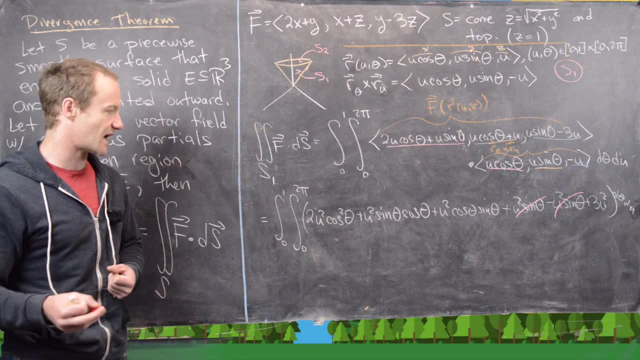 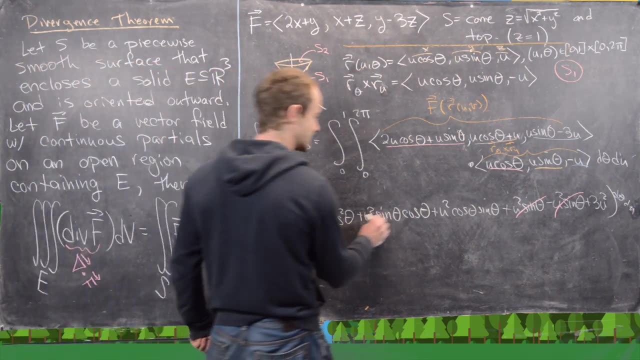 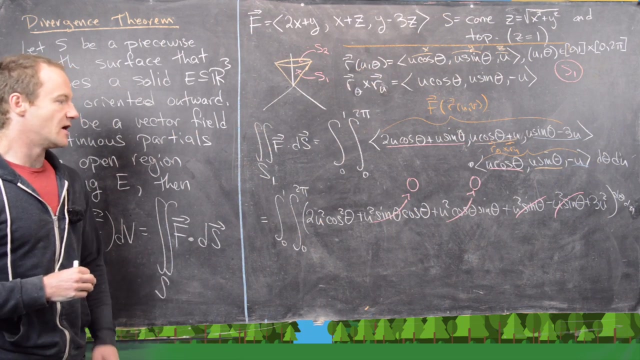 we'll do that with a U substitution. U equals sine, But notice sine evaluated at zero and two pi both give us zero. So that means this portion of the integral and this portion of the integral go down to zero. So you can check all the details for that. 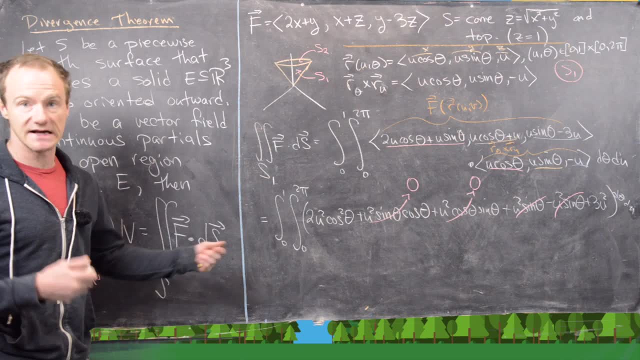 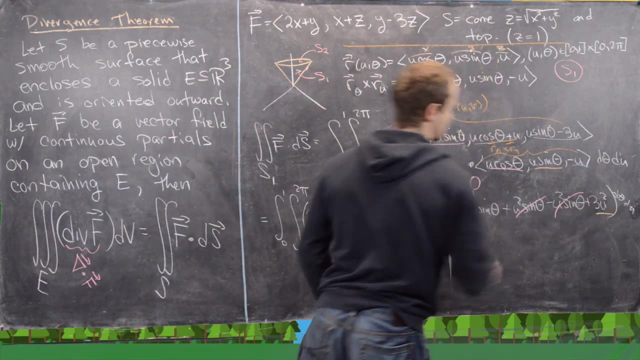 but that should be pretty straightforward, based on the fact where this lies, kind of within a multivariable calculus class. So, notice, all that we're left with is this term right here and this term right here, So I'm gonna go ahead and write that. 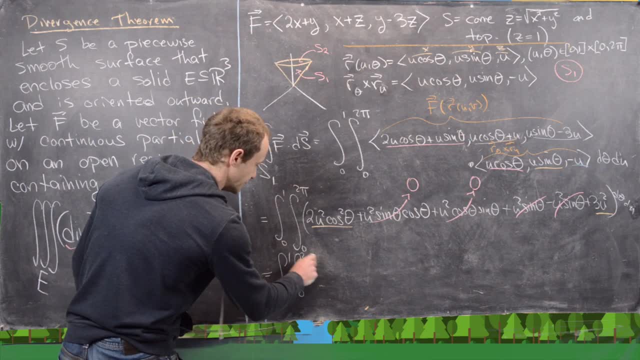 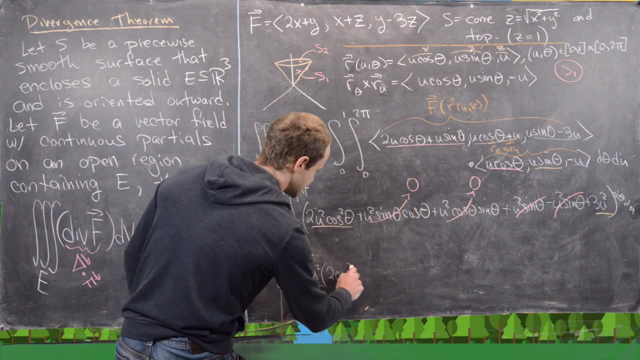 So here we have the integral from zero to one, the integral from zero to two pi, And now we have um, I'm gonna factor a U squared out of those. So we have U squared two, cosine squared theta plus three and then D theta. 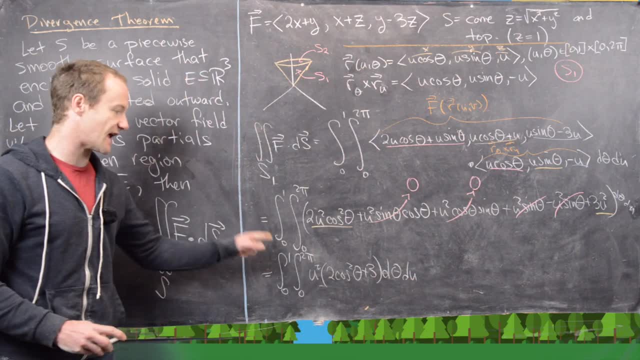 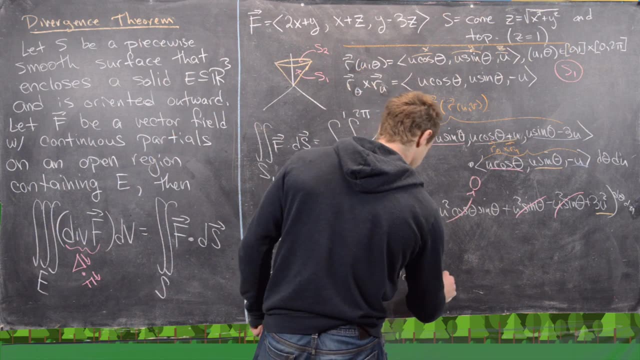 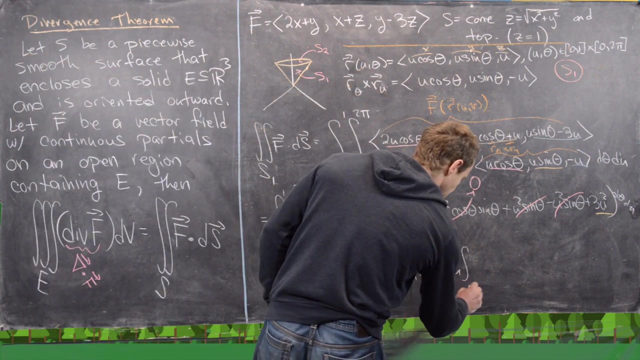 D U. But now notice that this is a function of U times a function of theta, So I can factor the integrals. This is going to be the integral from zero to one of U squared D U times an integral from zero to two pi. 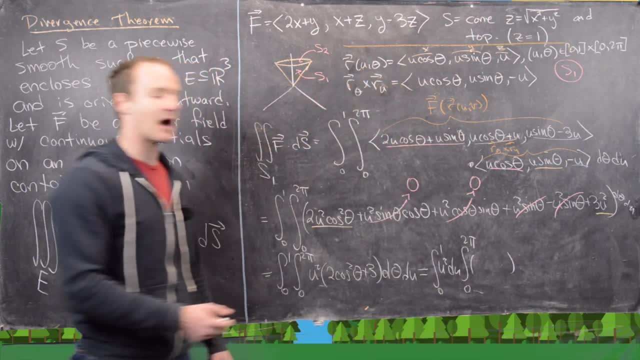 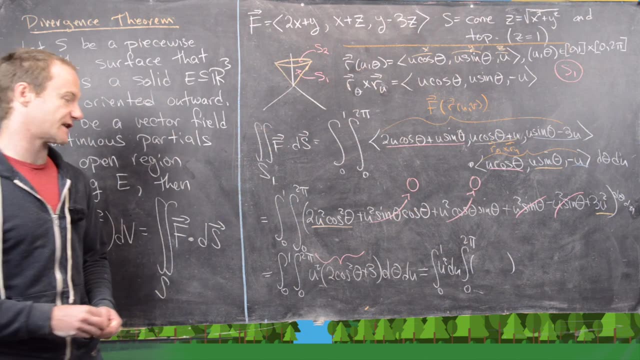 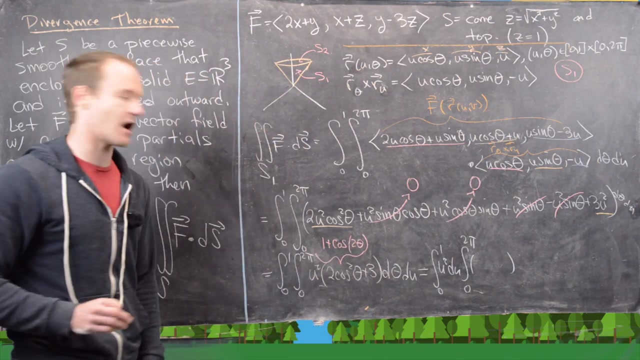 of the rest of that stuff, D theta. But I wanna rewrite that a little bit. I'll use the power-reducing formula to rewrite that two cosine squared theta as one plus cosine two theta Again, like this is a really common formula. 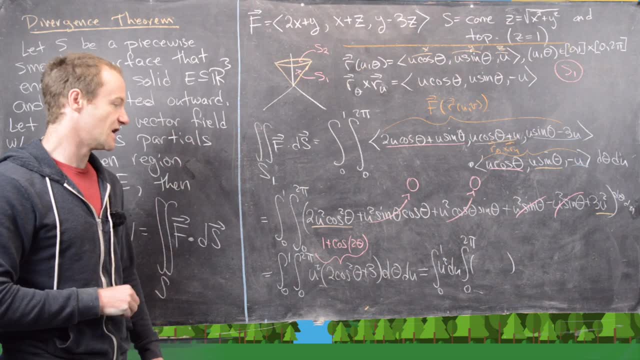 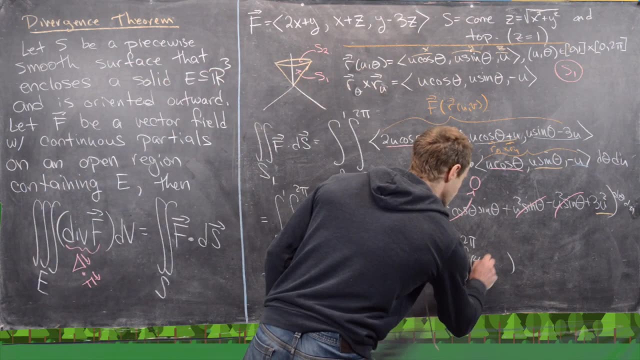 when we're doing these kind of triple integrals and surface integrals and stuff like that. So that's really useful to remember. Now we're gonna combine that one with that three to give us four plus cosine, two theta and then D theta. 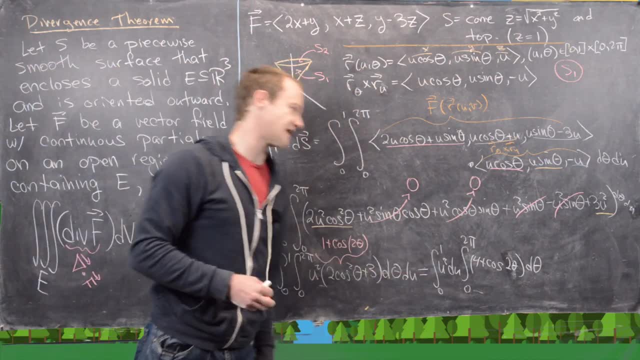 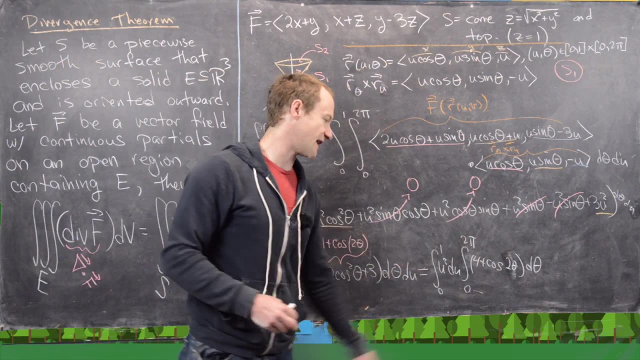 Okay, great. Now the next thing to recall is that when we take the antiderivative of cosine, we're gonna get sine. We'll actually have one half sine, two theta here, but we evaluate that at two pi and zero and that's gonna give us zero. 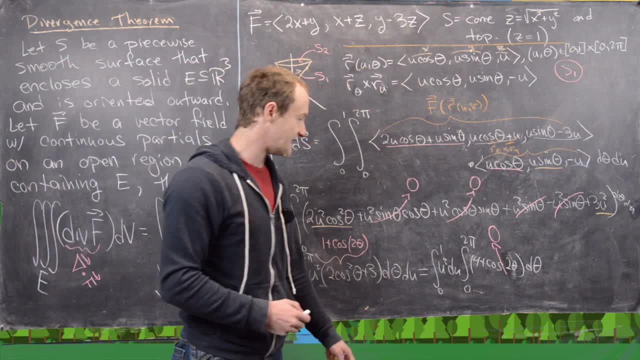 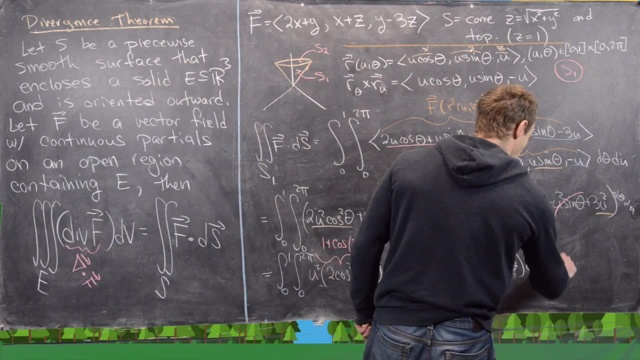 So this whole thing zeroes out And notice it's easy to see what goes on here. The antiderivative of that it's gonna be: U, cubed over three, evaluated at one, gives us one third. And then here we have four times two pi or eight pi. 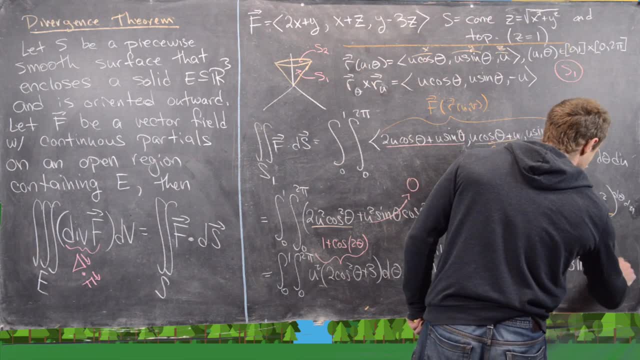 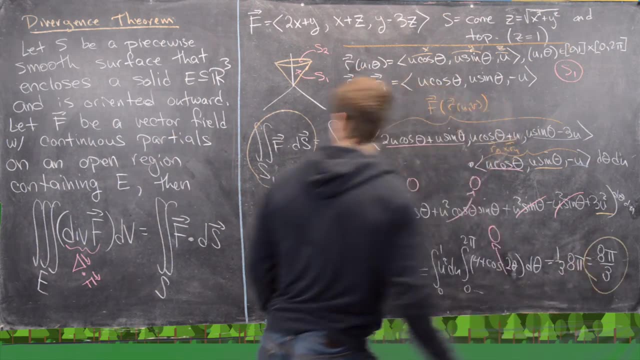 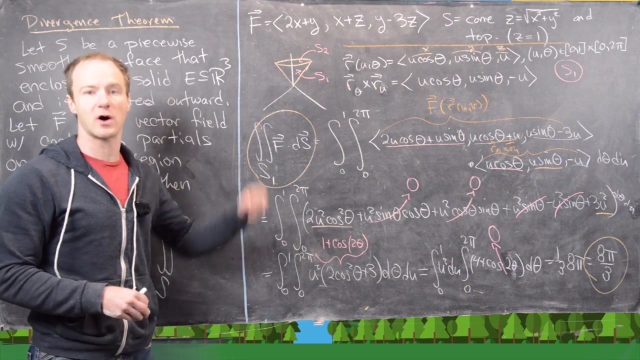 So one third times eight pi gives us eight pi over three Great. So our surface integral over the cone part of our surface gives us eight pi over three. Now we'll do the surface integral over the S two part, In other words the top of that cone. 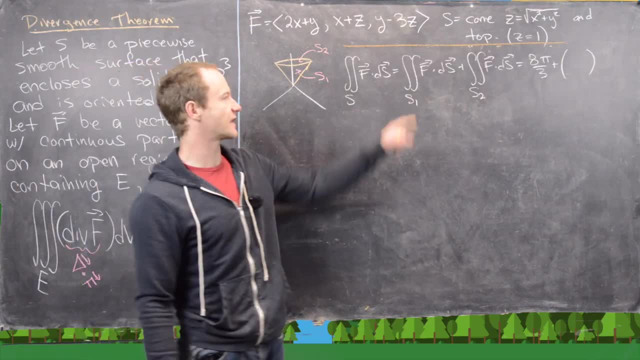 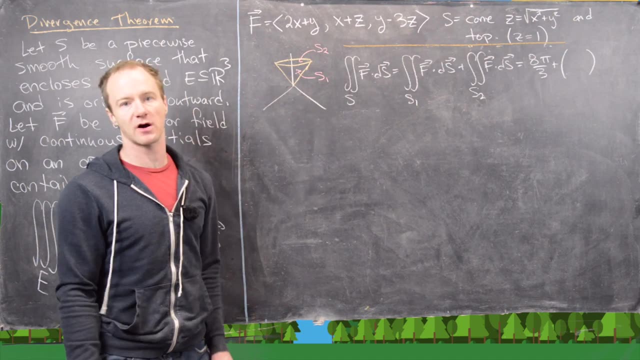 I'll clean up the board and we'll get to that All right. on the previous board we finished calculating the surface area over this S one, which is this cone part, not the plane on top, but the circular part on the sides. 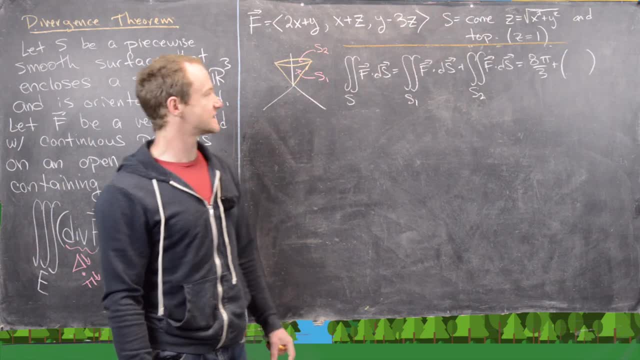 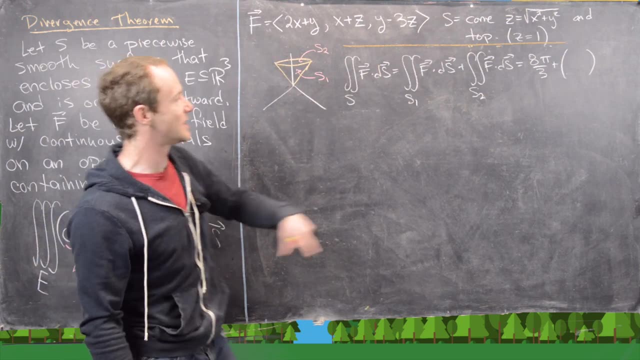 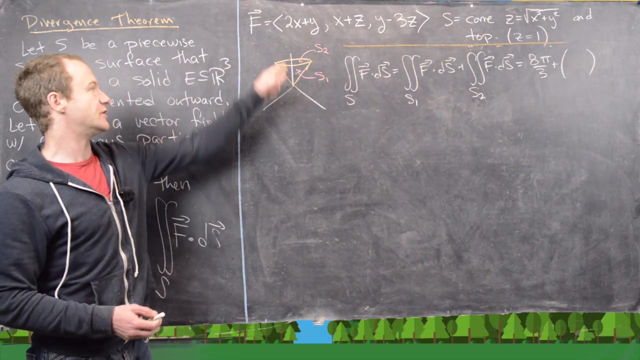 And we got that that was eight pi over three. So all that's left to do to calculate the surface integral of this whole closed surface is to calculate the surface integral of the top. So that would be the surface interval over S two. So that's what we'll fill in here. 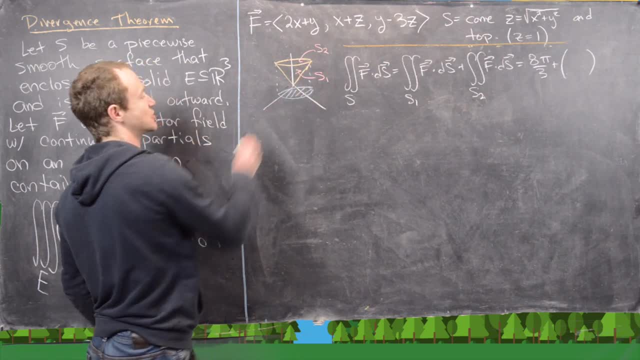 Okay, So the first thing that we need to do is parameterize this, But notice that this top healing, tasty сделera, as we know how to paramerize. So the first thing that we need to do is parameterize this, But notice that this top healing. 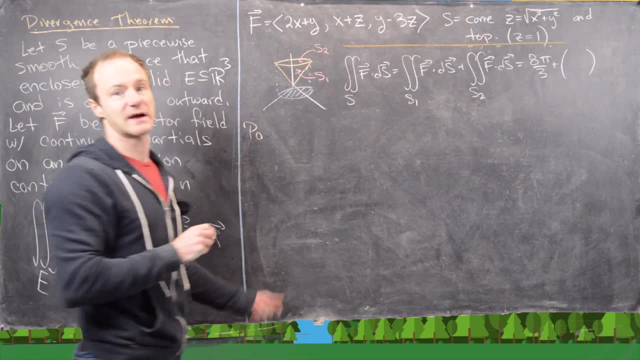 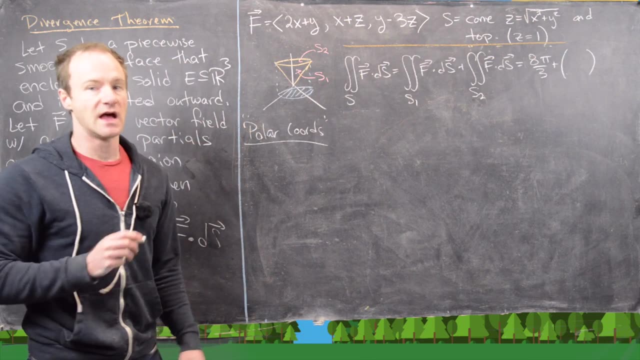 which we know how to parameterize down here in the plane. it's just that disk that's been lifted up. So we'll again inspired by some sort of coordinate system, and in this case we'll take inspiration from polar coordinates. And we'll do that to write R U theta. 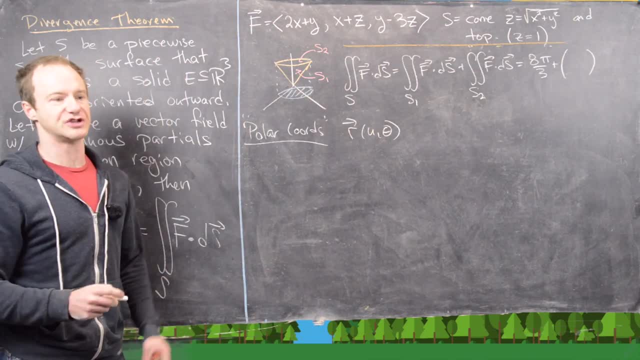 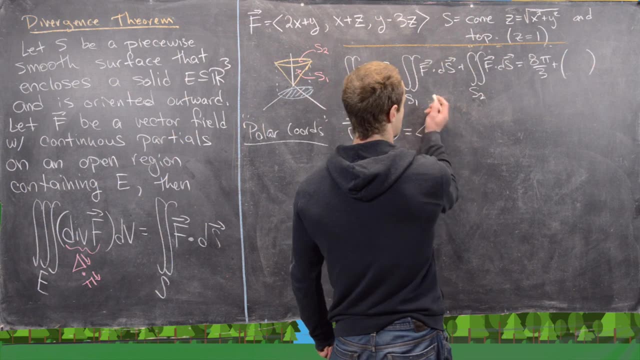 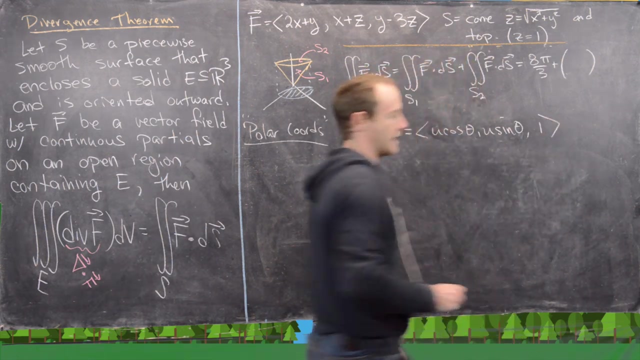 I'll take my distance from it. won't be the origin here, but it'll be the z-axis to be U, since we've already used R here. So notice this is going to be U cosine theta, U sine theta, and then comma one. 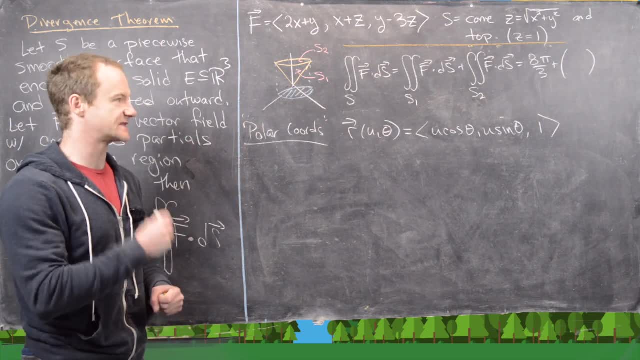 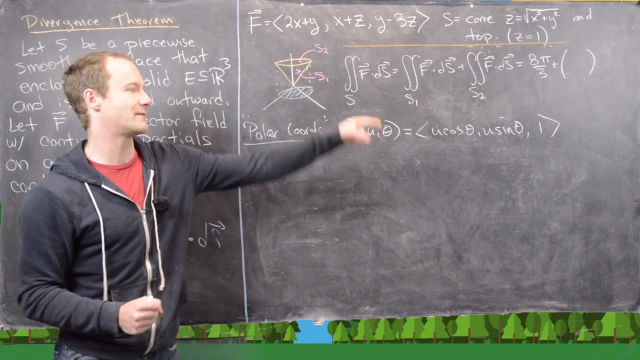 Again, notice: U cosine theta. U sine theta is like polar coordinates happening down in the xy plane. but then we boost that up to the plane z equals one by setting the z part equal to one. So that'll give us this disk up here. 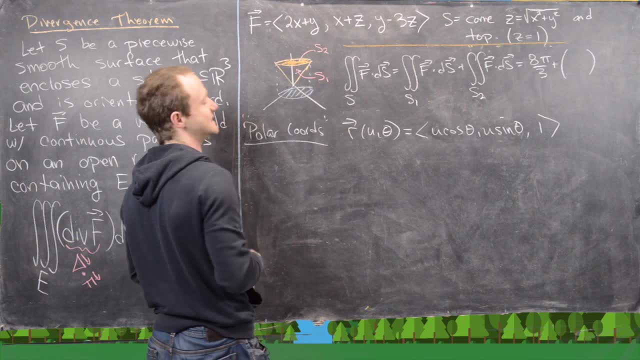 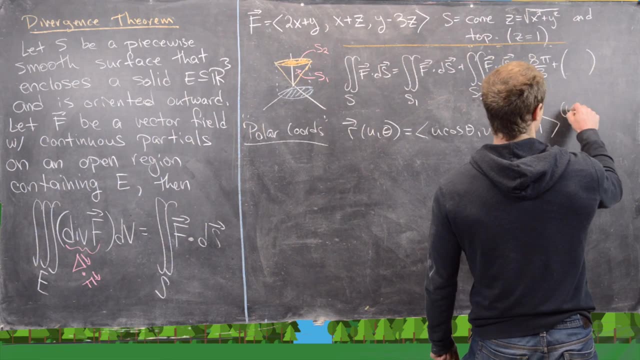 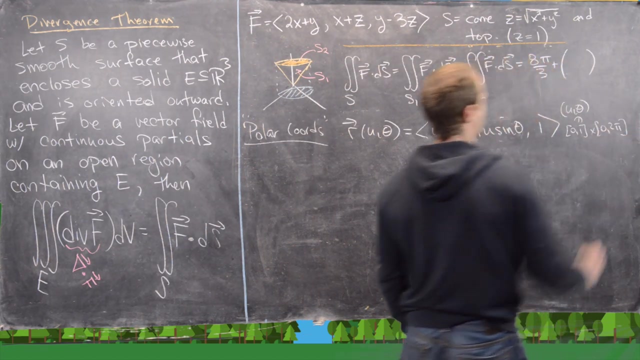 So, just to reiterate, we're parametrizing this disk, We're putting this disk up here being inspired by these polar coordinates, And now we can take U comma theta inside the cross product of the interval zero one, cross, zero, two, pi, kind of just like we did before. 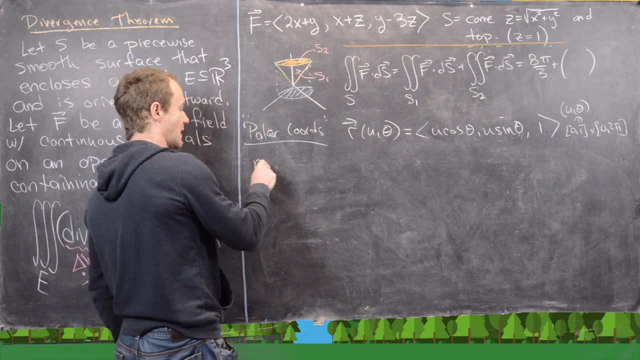 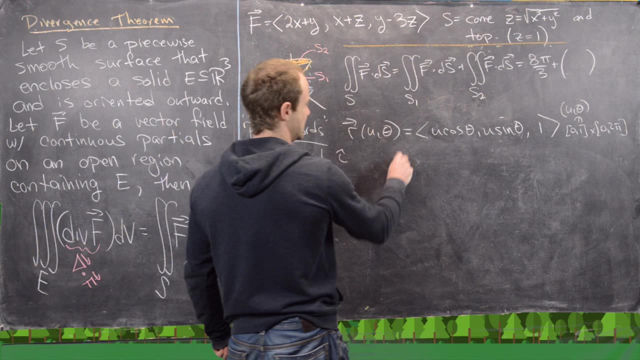 Okay, great. So now let's go ahead and calculate R? U cross, R theta. That's going to be an important part of this calculation, like we had before. So that's going to be. we need this cross product. we'll use the determinant version. 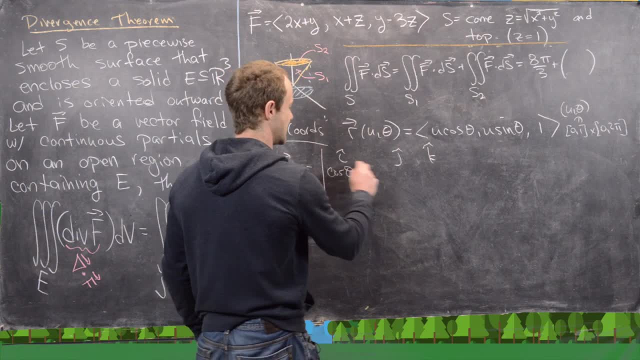 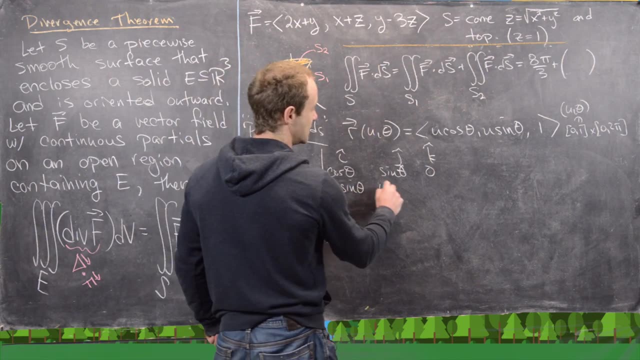 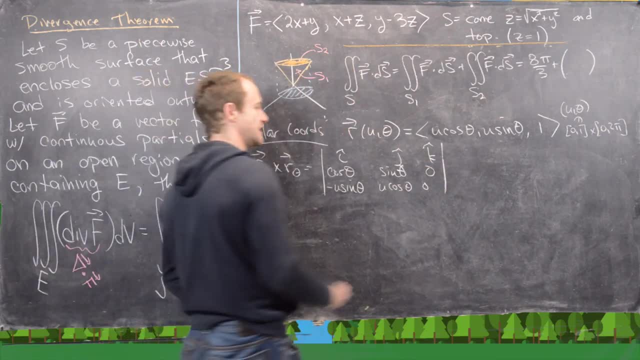 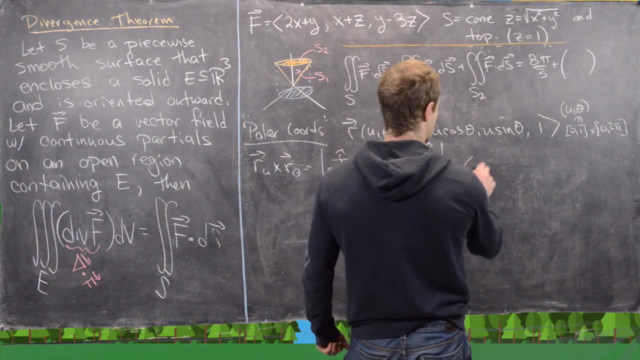 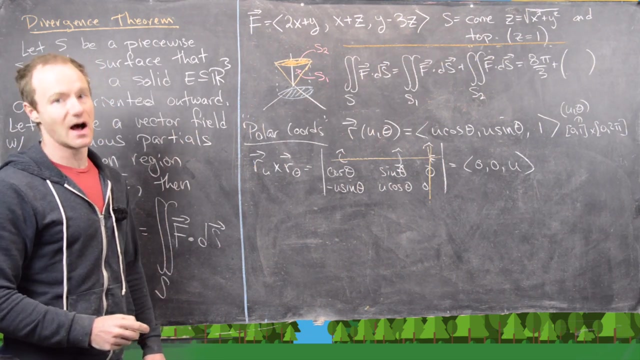 and then zero. Notice, the last component is the only non-zero component because of those zeros right there. So we'll get that from crossing these out and that will give us zero, zero U. Now we want to make sure that's pointing outward, but outward is upward in this case because 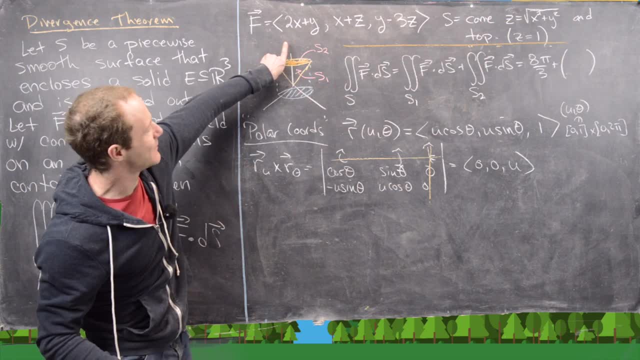 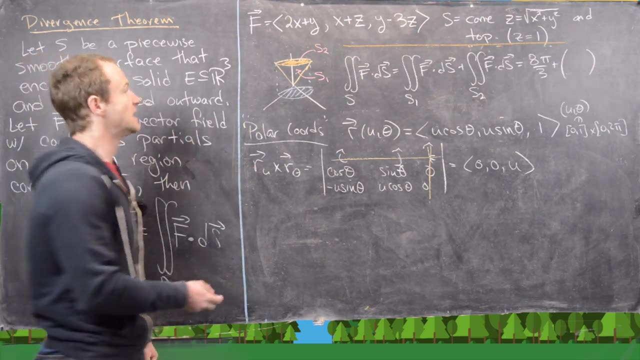 we're on this flat part of the top And, yeah, that's pointing upwards, because U is always between zero and one, so that's always pointing up. So we're good to go there. Now we can go ahead and apply our formula. 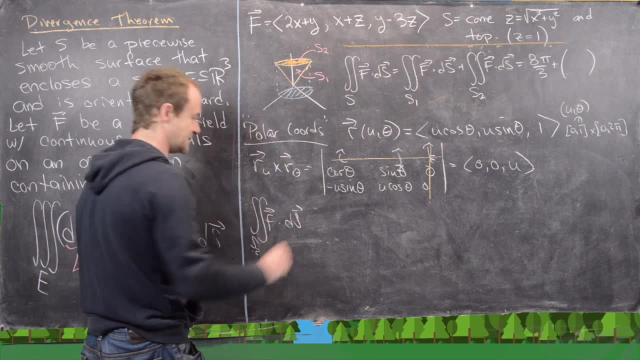 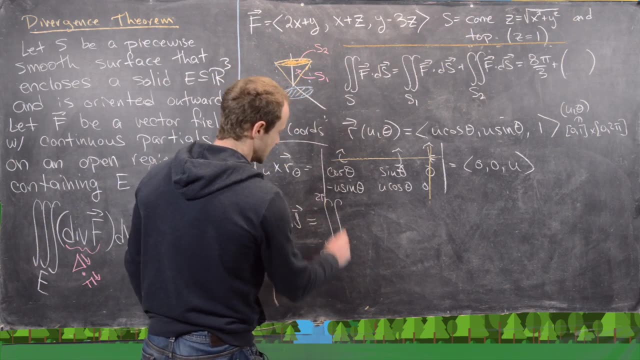 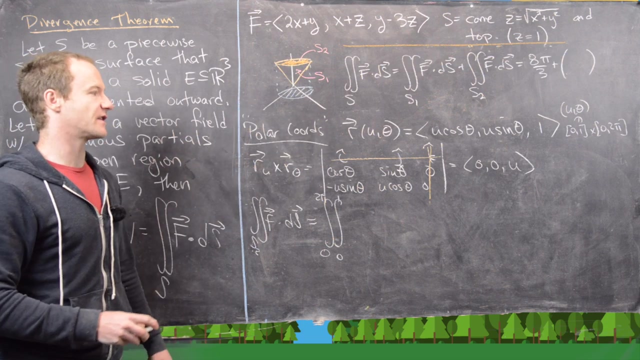 So the surface integral over S, two of F, dot, D, S, that's going to be equal to the double integral, zero to two, pi, zero to one. I should say iterated integral, because we know how to split it up. Okay, So we have F evaluated on the surface, but I'm going to use the fact that I'm going to 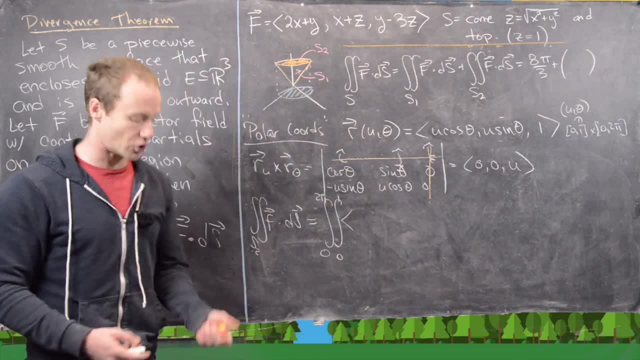 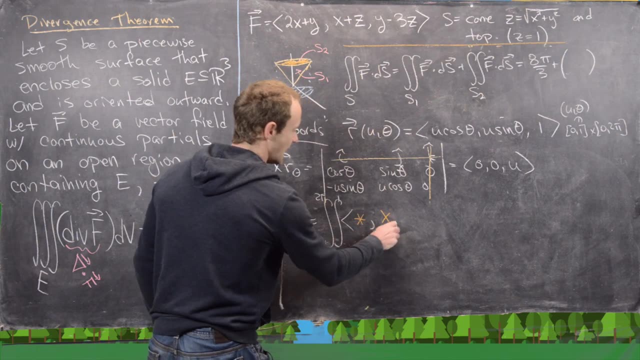 dot it into that, to point out that the first two components don't matter at all. So I'm just going to put asterisks there. So, like I said, those don't matter. And then comma: this Z component evaluated on the surface. 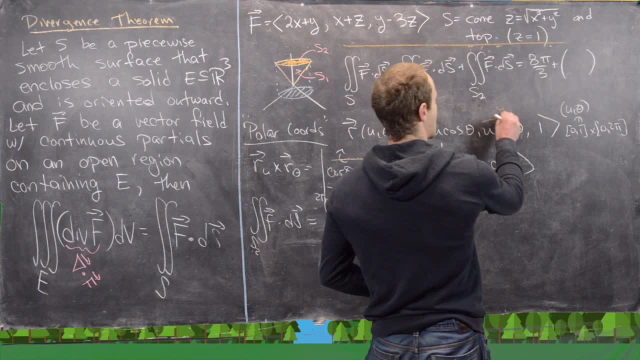 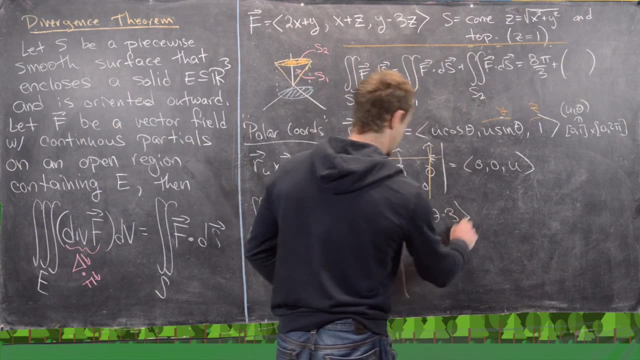 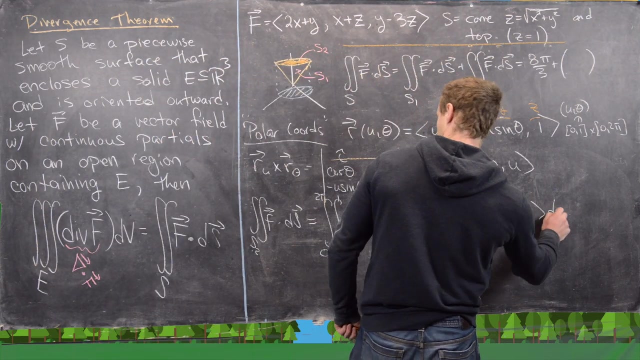 So we've got Y minus three Z, but we'll take this as the Y value and this is the Z value. So that's going to be U sine theta minus three. great, Now we're going to dot that into zero, zero U, and then we're doing this in the D U D. 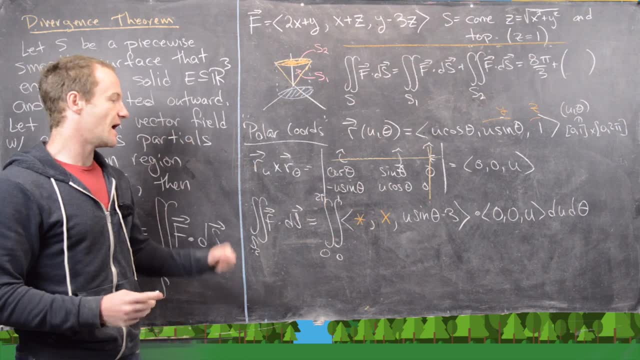 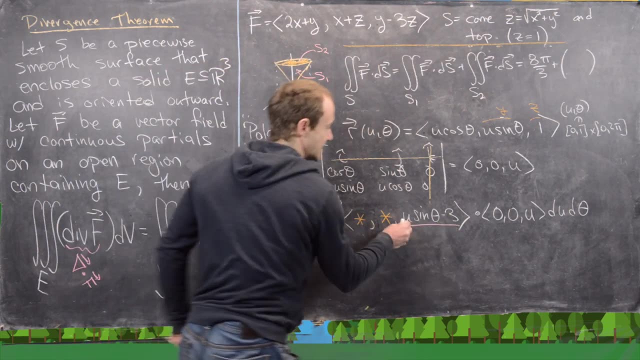 theta order. Okay, good, But, like I said, we didn't need these first two parts because we're dotting them into zero. So that doesn't even matter. All we need is this times that. So that's going to give us the integral from zero to two pi, the integral from zero to 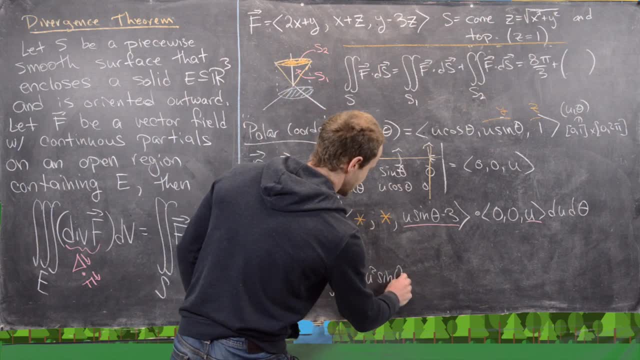 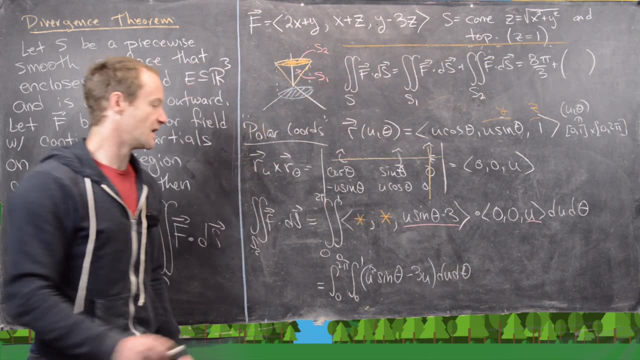 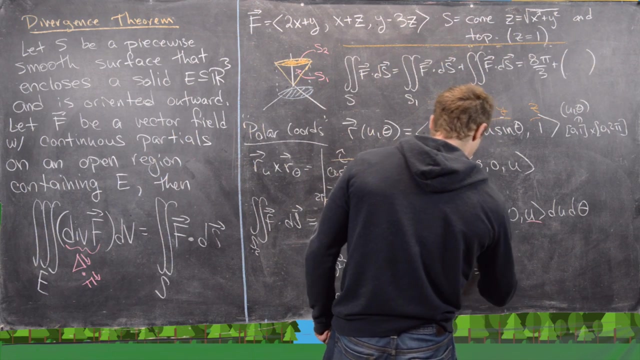 two pi and of. let's see, we have U squared sine theta minus three U D U D theta. Okay, Let's go ahead and take that U antiderivative first. So that's going to give us an antiderivative. sorry, zero to two pi, integral of theta on. 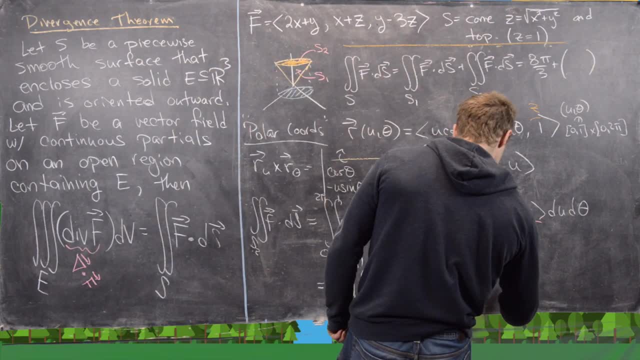 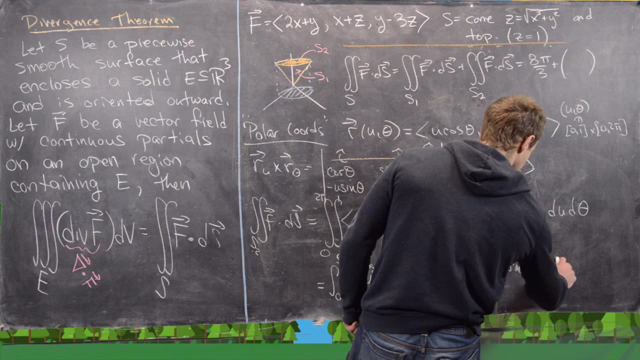 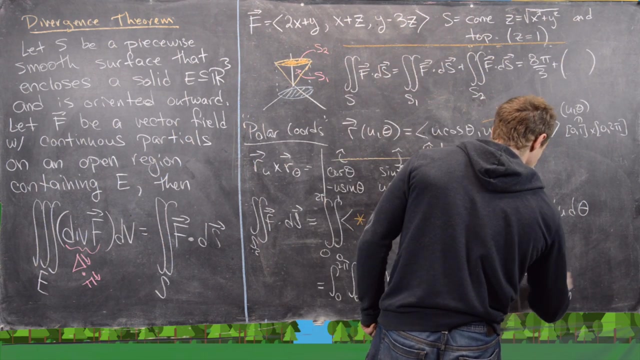 the outside. And now we have U cubed over three sine theta, minus three U d theta. Okay, And we're going to take that U antiderivative first, 3 over 2, u squared, and then we need to evaluate this from u equals 0 to u equals 1. 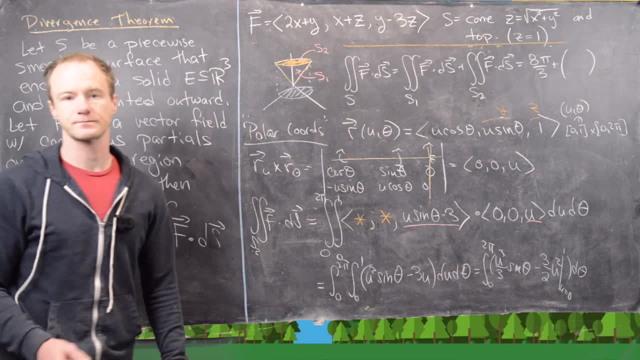 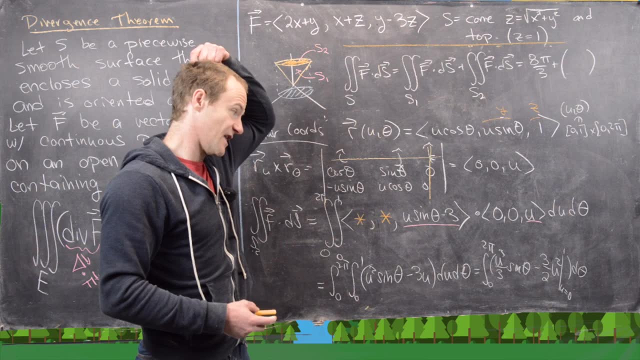 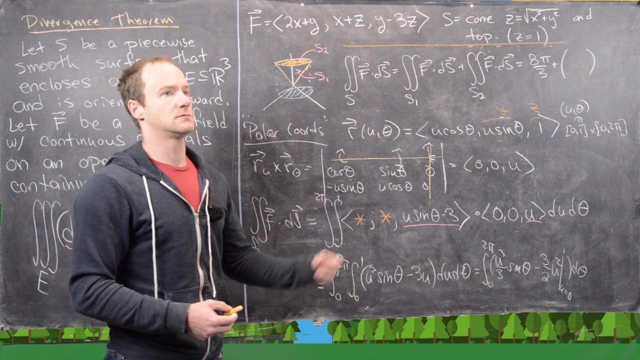 and then do a d theta integral. okay, so I want to cheat a little bit again. I want to notice, first off, that in this case, once we get around to the theta integral, we're going to be integrating sine over a whole period, which makes this sine part. 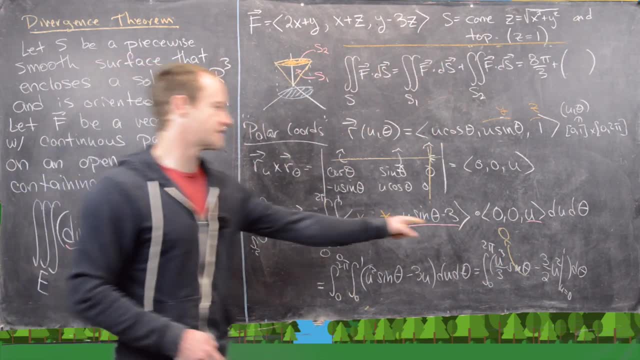 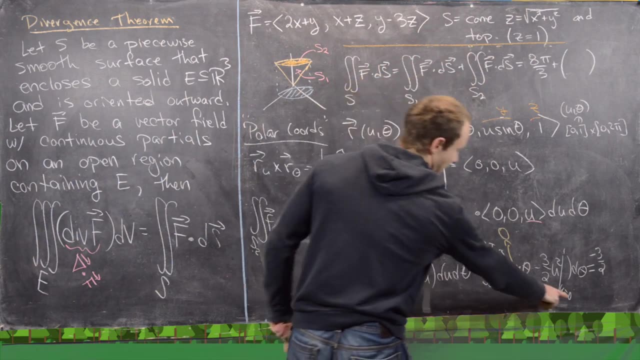 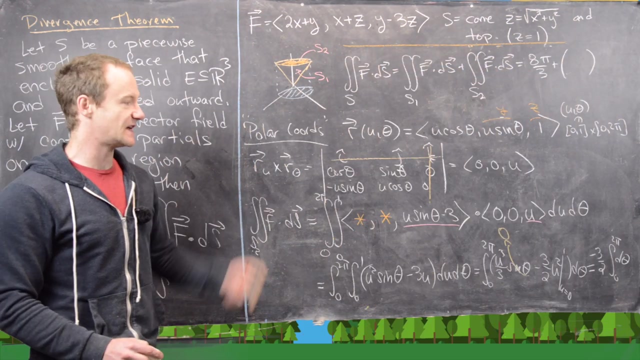 0 once we get around to the theta integral. so all we need to do is this: in the end, which is going to be minus 3 halves notice if we plug 1 into that and then the integral from 0 to 2 pi d theta. but now if we take the antiderivative of that and evaluate it at 2 pi, 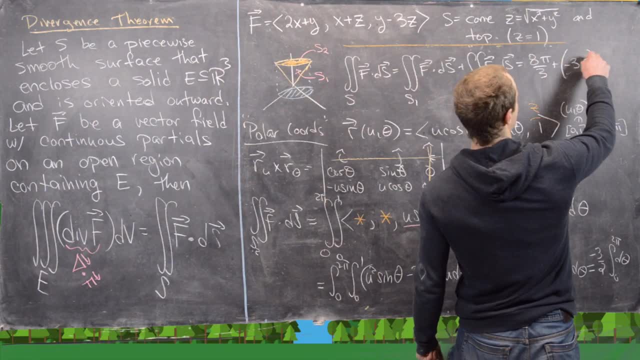 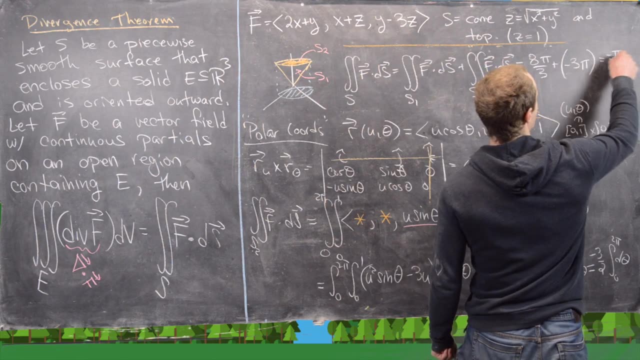 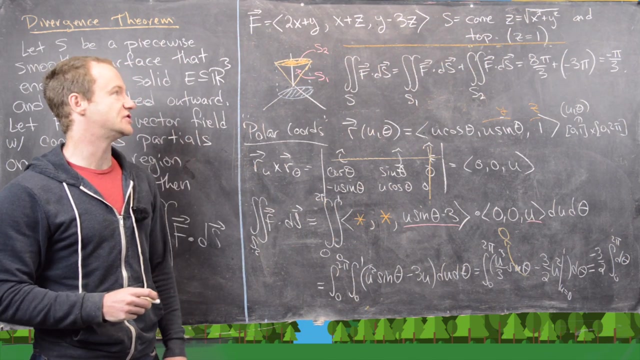 it's pretty easy to see that we get minus 3 pi. but now minus 3 pi is the same thing as minus 9 over 3, so this is minus pi over 3. so that is the total value of our surface integral. okay, great, let's go ahead and clean this up and then do the triple integral part.